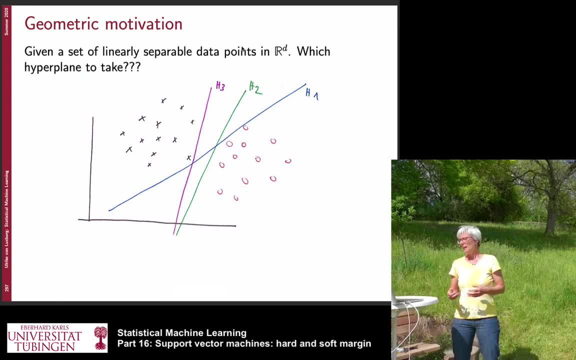 also for linear discriminant analysis. And again, if you look at the slide, we have the question: there might be many different hyperplanes that realize a particular classification of our data set. Now, which hyperplane are we supposed to choose? And we have already seen two different answers to this question. 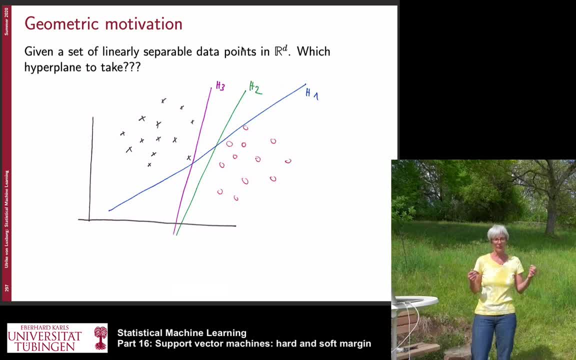 We have seen the geometric answer by linear discriminant analysis, where we said: you know, we need to project such that the classes, the points within the class, are projected tightly together and the distance between the classes gets very large. This was a geometric motivation. 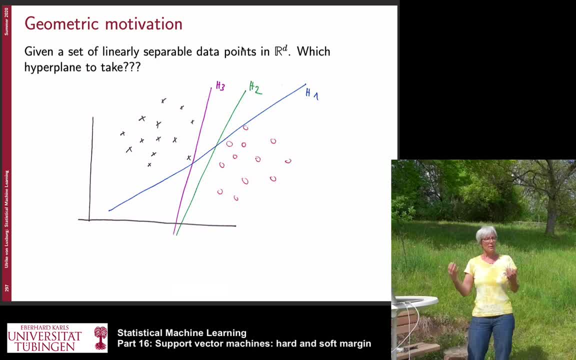 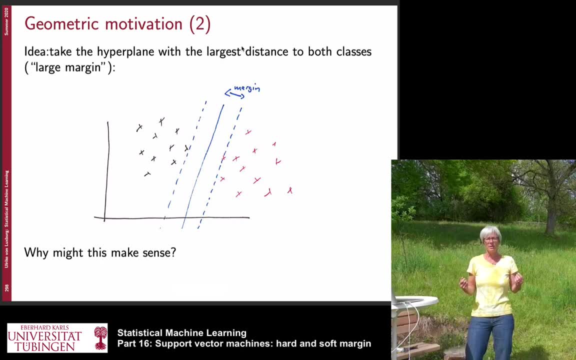 And now we want to see another geometric motivation, the one that leads to support vector machines. in the end, The main idea of support vector machines from a geometric point of view is what is called the margin. So consider the slide and assume we have a data set that is very nicely separable by 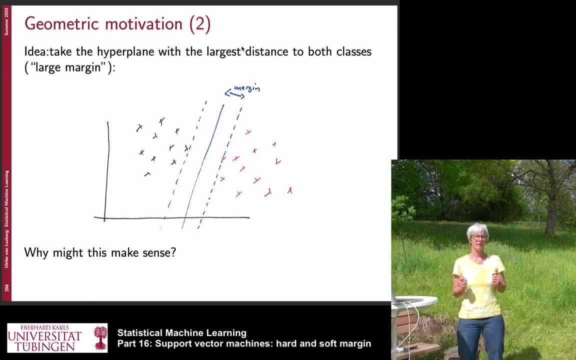 a hyperplane. So there exists a hyperplane that can perfectly separate all these data points from each other, the points from the two classes. Now, if there's one hyperplane, there are often many hyperplanes that can separate the data. And now, which one are we supposed to take? 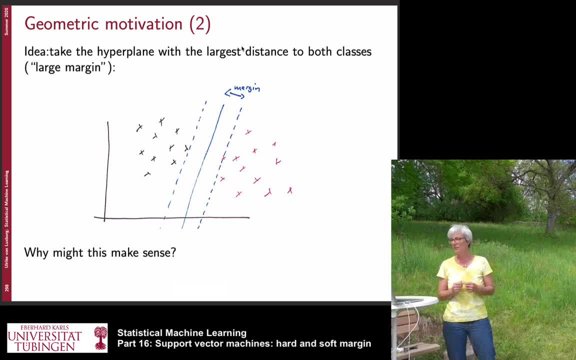 What we do is we consider the margin, And the margin, as you can see it here in the plot, if you have a hyperplane, you sort of draw the margin. You go in parallel to your hyperplane outside from your hyperplane as far as you can go. 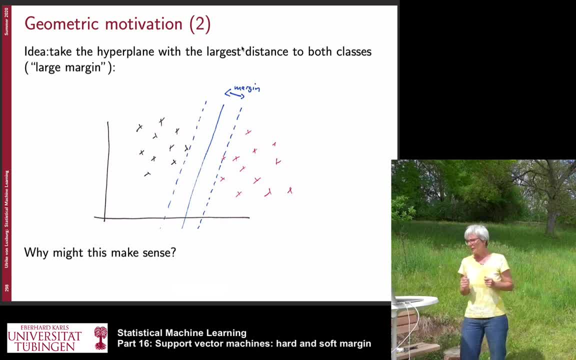 before you touch a point. You can see that on the slides. So the hyperplane is somewhere and then sort of the margin is where, like if you go to the outside, where you start touching the points from the two classes, And the idea is we would like to find a hyperplane that has a large such margin. 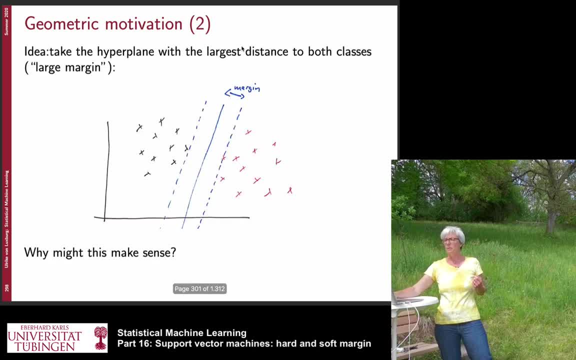 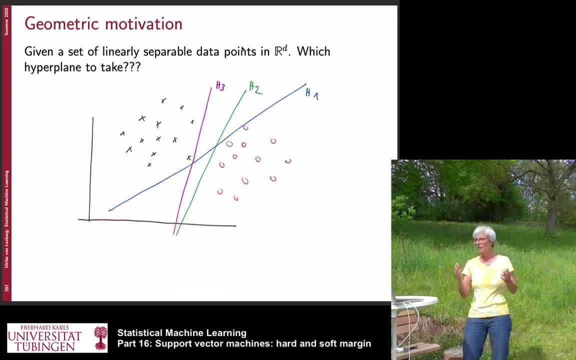 I would maybe like to go back to this example we had on the previous slide. If you consider the three hyperplanes here, you might want to say H1, sure it classifies all points correctly, but it is very close to the red class. 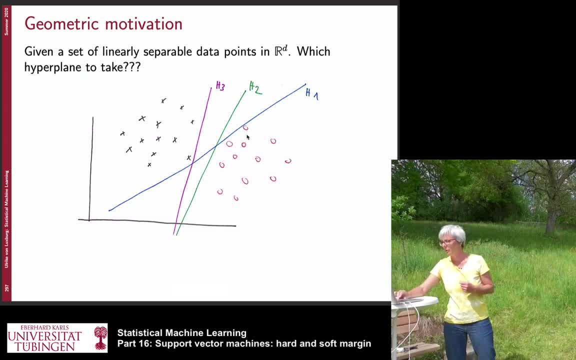 I don't know whether you will be able to see this in the video, but here, at this particular point on the right top of the plot, the hyperplane is close to touching this red point And if you now imagine, if you add a bit of wiggling to this red point, for example, some 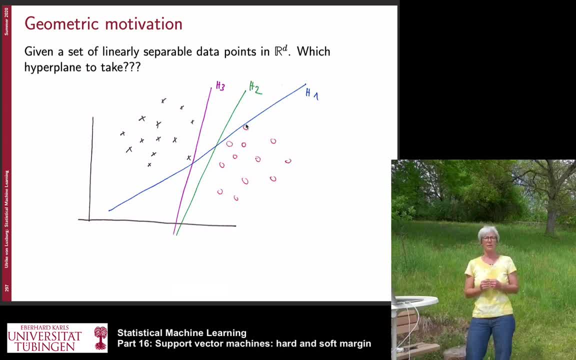 measurement noise, then it immediately might jump to the other side of the hyperplane and might get a different label. So in this sense, if you would choose the hyperplane H1, it doesn't seem like a pretty robust choice. If we add a little noise to our data, the classification of some points might change. 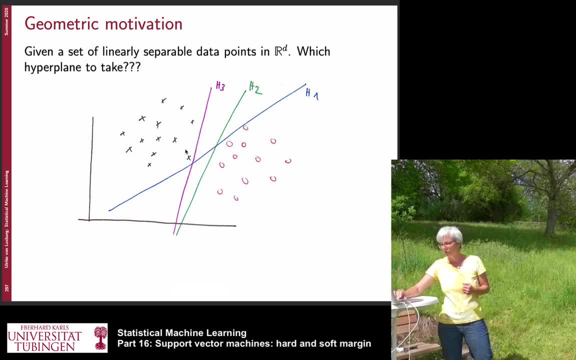 The same is true for the hyperplane H3. So here this is close to this other data point here from the other class, And hyperplane H2 is at least a bit better because its distance from the two classes is a bit larger, If you only add a tiny amount of noise to your training points. the classification of 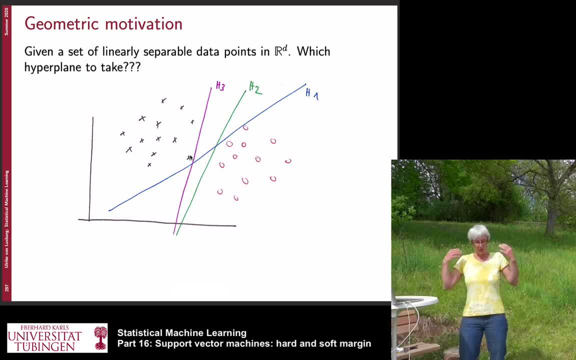 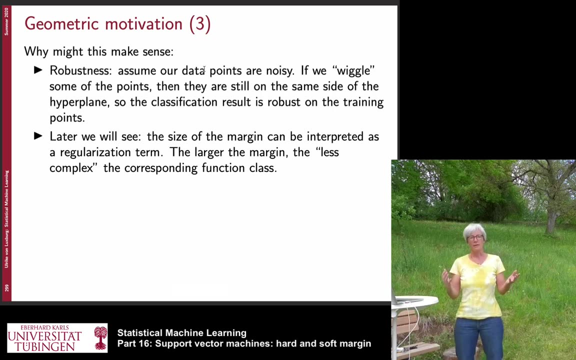 these training points is not going to change. So this is one of the reasons why we would think that having a large margin might be a very good idea. It adds some robustness to our classifier. So one of the reasons why we might want to have a large margin is robustness, because 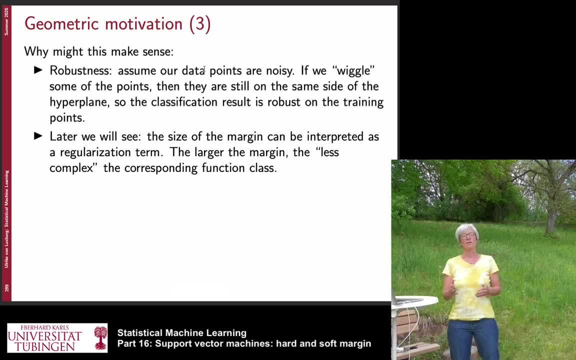 if we add a bit of noise to our data, the classification of the data points might not change as easily. What we are going to see later on is that the size of the margin also induces some kind of regularization, And the larger the margin, the higher we regularize. 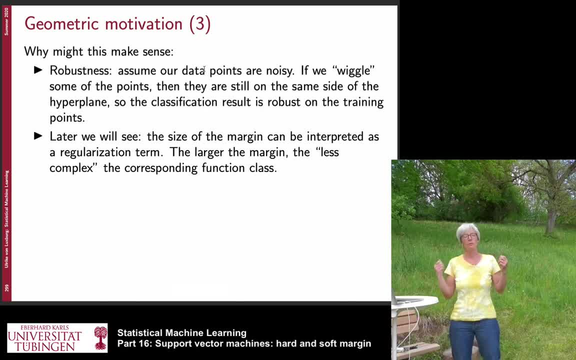 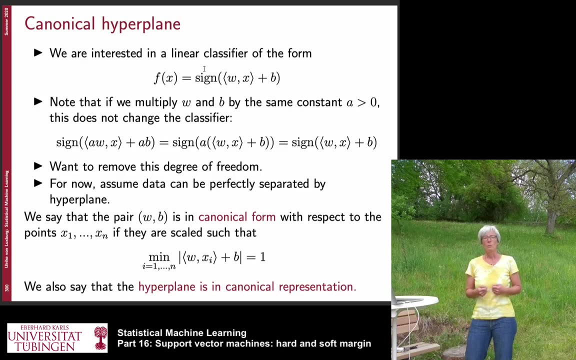 And if we manage to find classifications or if we find functions that realize a separation with a large margin, this means that we have found a very simple function from a small function class. But this is going to come later. Let's get a bit more formal. 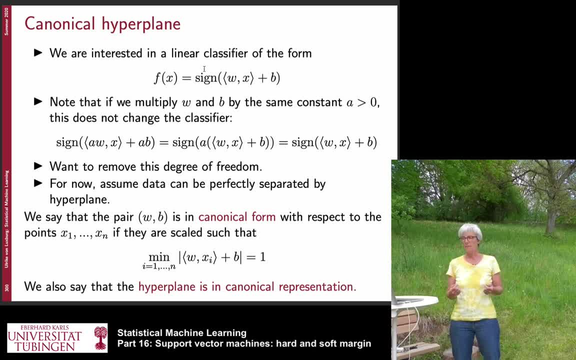 What we want to do is we want to do classification by a hyperplane. So what we are interested in is a linear classifier of the form that we have seen before, a function that is the sine of omega, x plus b, where omega and b are the two parameters that we 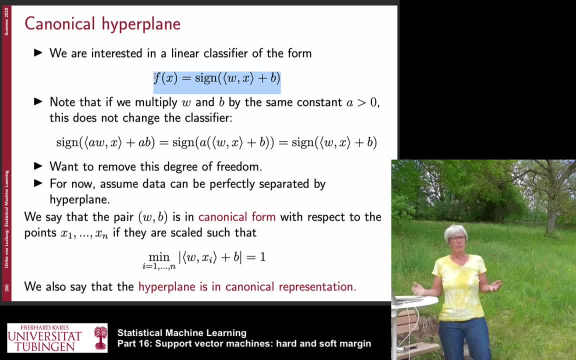 want to learn For the SVMs, if we want to solve an optimization problem. there is an important thing that we need to figure out right now, Namely, if we multiply the parameters w and b by the same constant a, then of course the 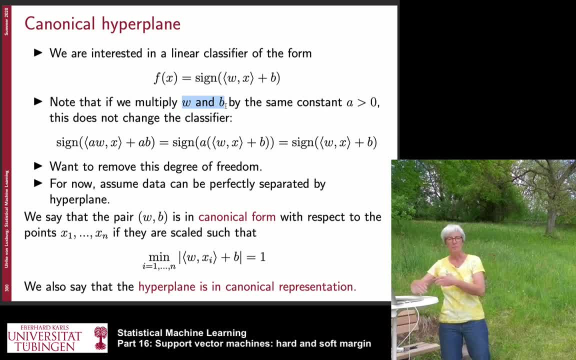 hyperplane is not going to change Because if you look at what happens to the sine of this function, it is still the same. So if you look at here the sine, like here, I multiply it a times w and a times b and 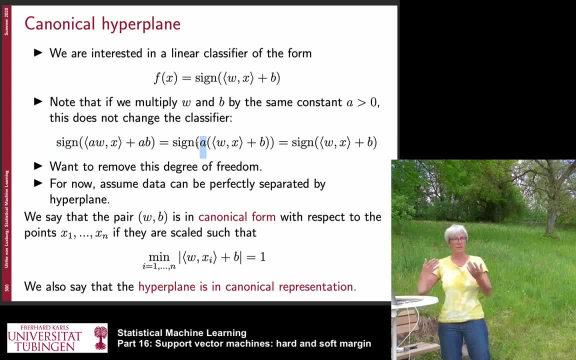 then I take the sine- and of course you can take a out, because it's a linear function- and then the sine. if a is a positive constant, the sine doesn't have any influence on the sine of this function And this, but this is a degree of freedom that one often wants to get rid of in optimization. 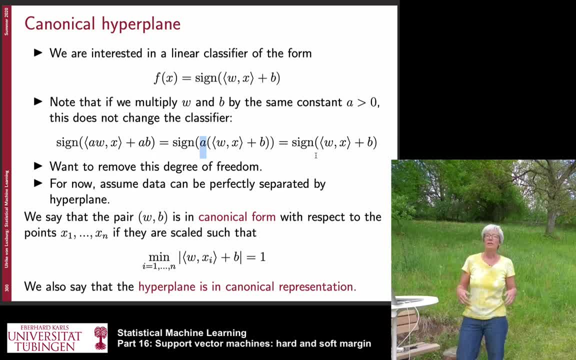 problems, Because often this degree of freedom sort of hinders you to find a good solution for your optimization problem or the it's sort of it's one degree of freedom that you don't like to have. So what we, what you typically do in such a situation? you fix some constant that you 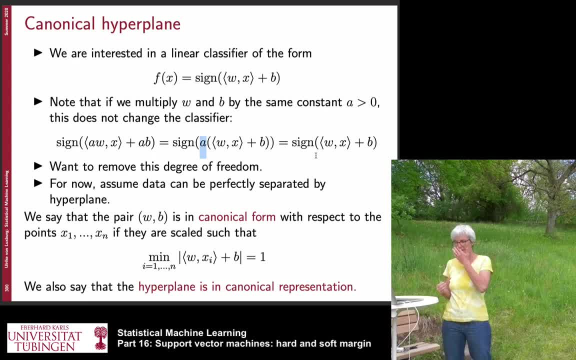 want to take And the way we fix it in this particular case is: we define what is a hyperplane in canonical representation or in canonical form, And here is the definition. We say that the pair w- b is in canonical form, And here is the definition. 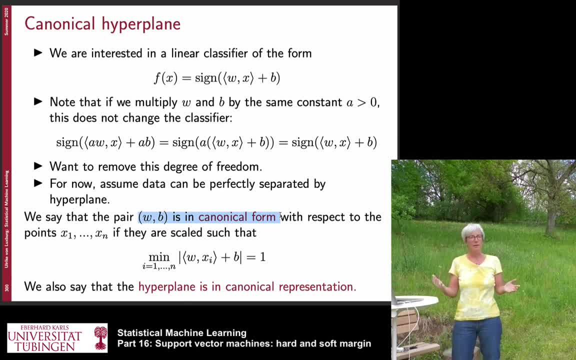 We say that the pair w b is in canonical form, And here is the definition. We say that the pair w b is in canonical form With respect to the given data points that you have. if the following is true, you evaluate: 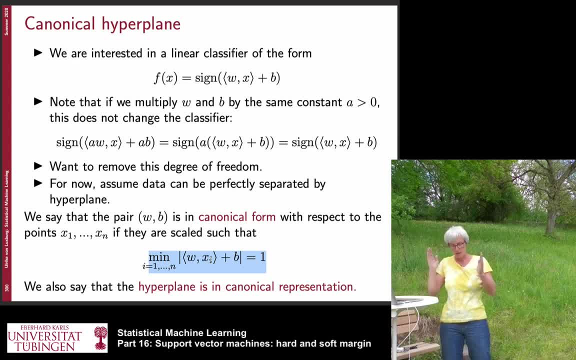 the absolute value of w, like of of the hyperplanes on your training points. So w x, i plus b is the value that this hyperplane function takes on all your training points. Now we're only interested in the absolute value and we want that the minimum of these. 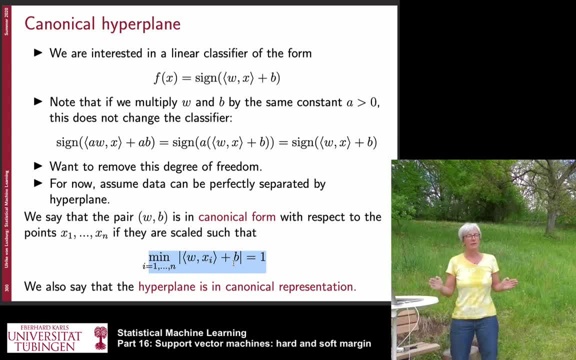 absolute values is 1.. And this fixes implicitly the constant, the constants, because if we would now multiply this by a constant, then the minimum would not be one anymore. So we choose essentially the constants by which we could multiply in omega and b, by 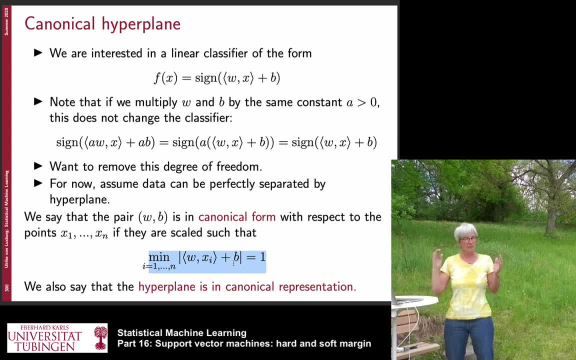 fixing it such that this equation is true. And if this equation is true, then we say we have a hyperplane in a canonical representation. This is some kind of ad hoc notation. it's only used in support vector machine. This is nothing that you would see somewhere else in mathematics or so, so this is just. 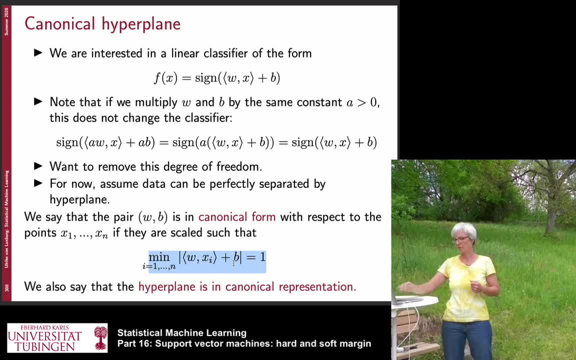 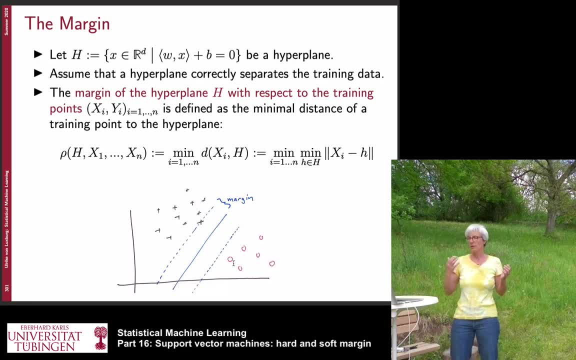 used a term which is helpful for support vector machines. Now let's try to formally define the margin. So again, we say H is any hyperplane, and for now we assume that we have a training set and that this hyperplane perfectly separates this training set. 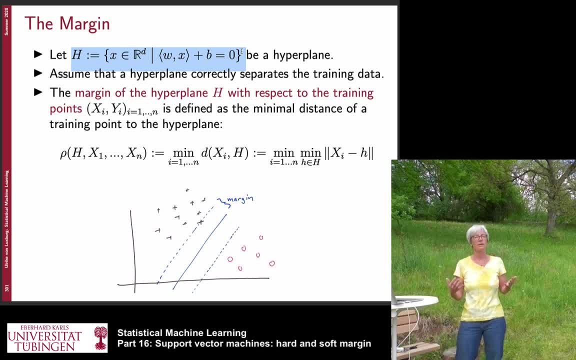 So we start by introducing support vector machines in the perfectly realizable case. Now we want to define what the margin is And we say the margin of the hyperplane H with respect to the given training points is defined as the minimal distance of the training points to the hyperplane. 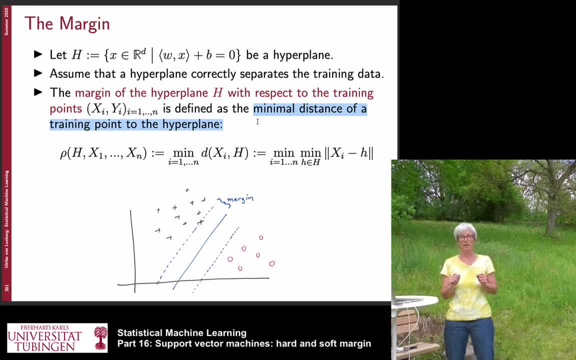 So for each training point you compute what is the distance of the training point to the hyperplane, and then you take the minimal distance, and this is then what we call the margin, And recall this sort of corresponds to our intuition. the margin somehow measures by. 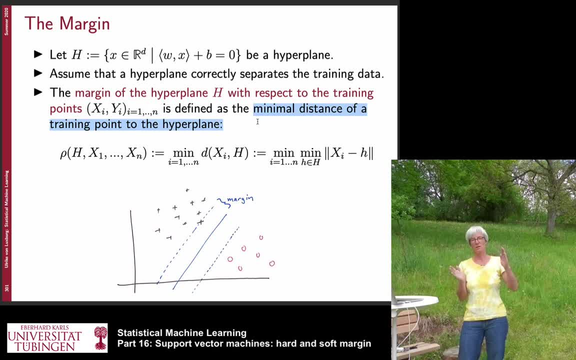 how far I can move the hyperplane. a step start to touch the training points and this is exactly the distance the training points have from the hyperplane. So the formal definition rho, the margin in the support vector machine literature is always called rho. rho of the hyperplane with respect to the training points x1 to xn is: 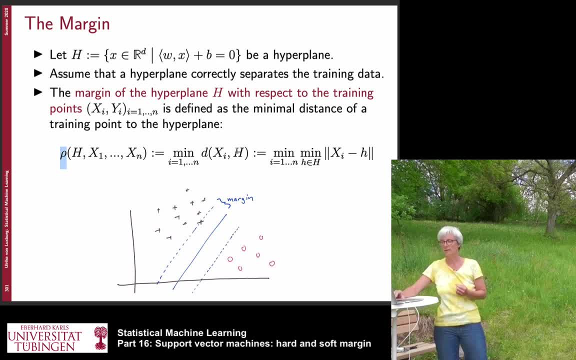 defined as the minimum distance of the training: points xi to the hyperplane. And now if you look at what is the distance of a point to a hyperplane, the distance of a point of point xi to the hyperplane is just you check for all points on the hyperplane. 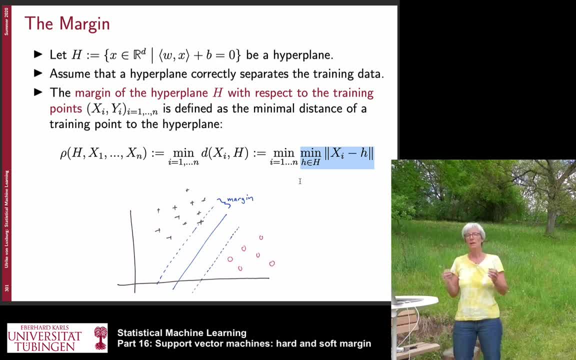 which one is the one that is closest to the training- point xi- and then you take the minimum over all of those and this is the distance of a point to a hyperplane. Okay, and in the image again, if you look at it, we have the two classes, we have the hyperplane. 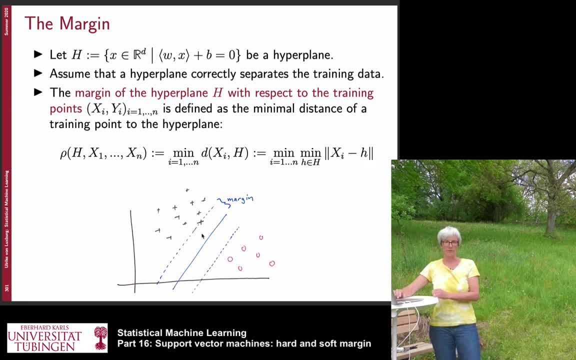 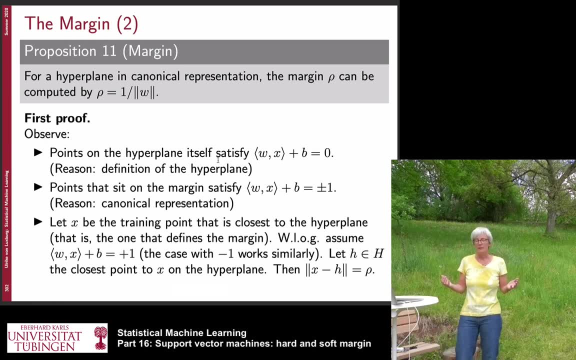 and the margin is the distance of the hyperplane to the closest training point. Now the first proposition we want to make is how to compute the margin given. we have the hyperplane and we have the training points. And the proposition now says: for a hyperplane in canonical representation, the margin rho. 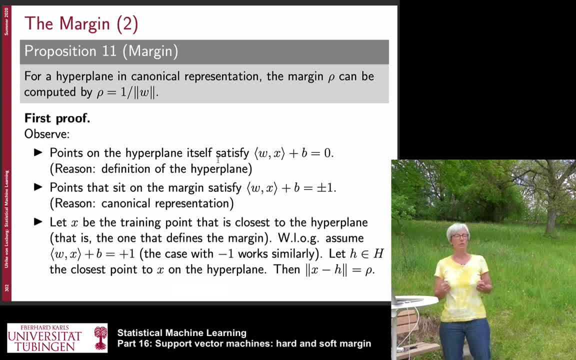 can be computed as rho is 1 over the Euclidean norm of w. So we are still in the Euclidean space because we do linear classification in the space Rd. We look at the Euclidean norm in this space and the norm of w. 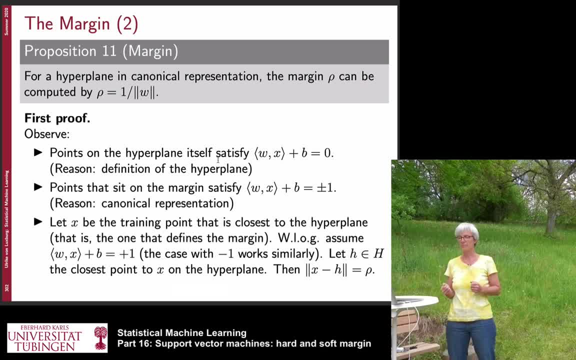 The inverse norm of w is: what is the margin. and there are many different ways in which you can prove that, and they are all very simple, but I want to show you one of them. It goes as follows: So assume we have a point on the hyperplane, so x is a point that sits on the hyperplane. 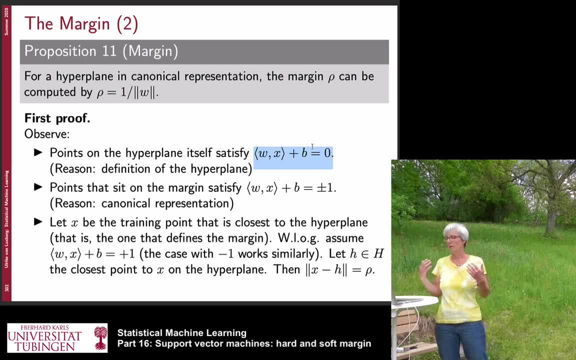 Then obviously it has to satisfy the hyperplane equation, which is wx plus b is 0.. So this is just by the definition of the hyperplane. Now, if we have a point that sits on the margin, We know that this point satisfies omega. x plus b is either plus 1 or minus 1.. 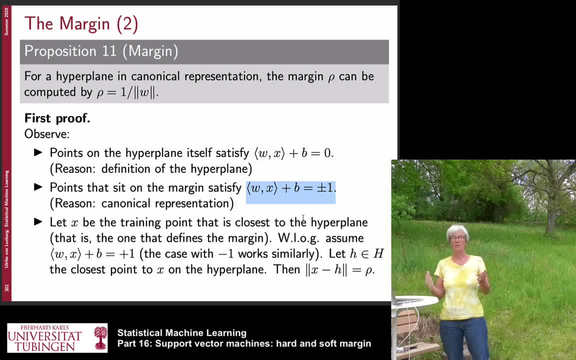 And this comes from the definition of the canonical representation and from the definition of the margin. And now we consider x being the training point that is closest to the hyperplane. So there might be many training points, but we look at the one that is closest to the 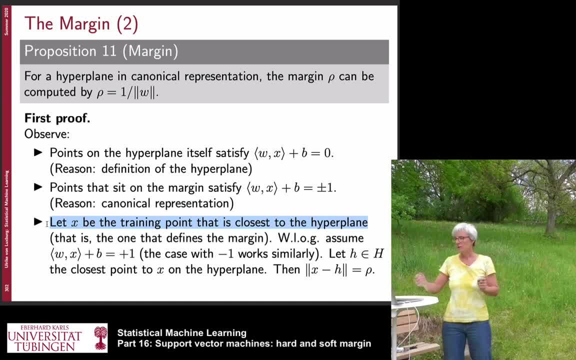 hyperplane And without loss of generality. We now assume That it takes the value plus 1, so it could be minus 1 or plus 1.. The argument goes exactly the same way. you just have to change the sign. 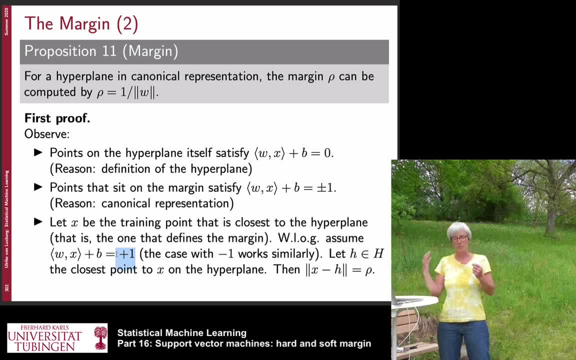 So, without loss of generality, we use plus 1 here And now let h be that point on the hyperplane which is closest to this point x. So we now have x as this point that is closest to the hyperplane. So here we have x, here we have the hyperplane. 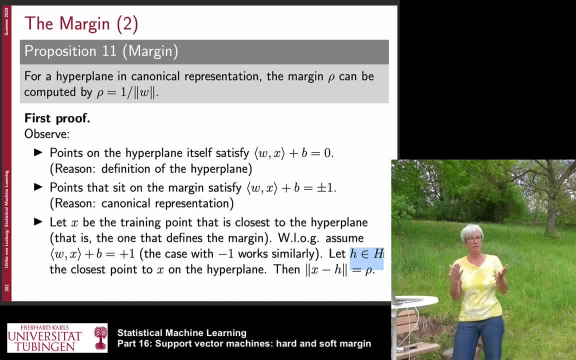 And here we have this point, lowercase h, which is the point that is closest on the hyperplane, which is closest To x. And now, by all the things we have defined above, it's easy to see that the distance of x to h is rho by the definition of the margin. 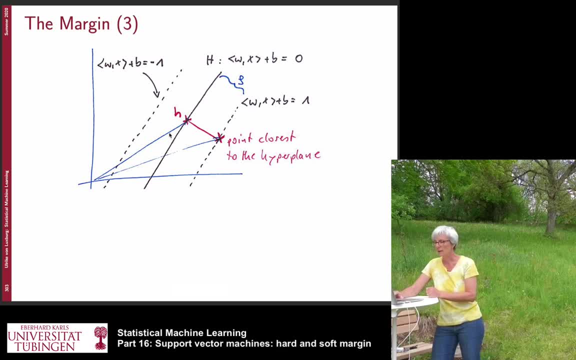 And here is a figure maybe to illustrate it. So here we have, in the middle we have, the hyperplane Which satisfies omega. x plus p is zero. Here we have this point, that is the red point here, which is closest to the hyperplane. 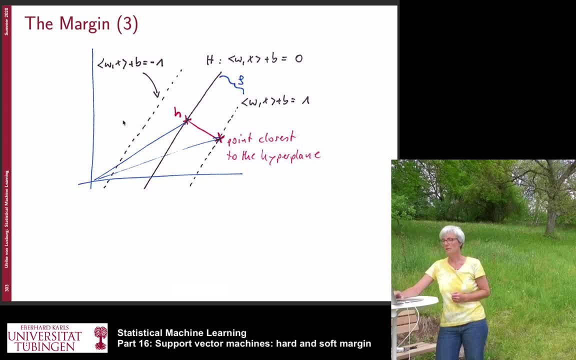 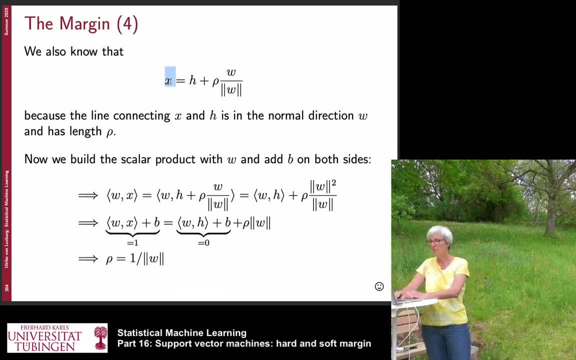 And it satisfies: omega x plus p is 1.. Points on this other side would satisfy: omega x plus p is minus 1. And we're interested in this distance here. this is the margin, which is rho. Now, what we also know is that x, the point x, can be written as h plus rho times omega. 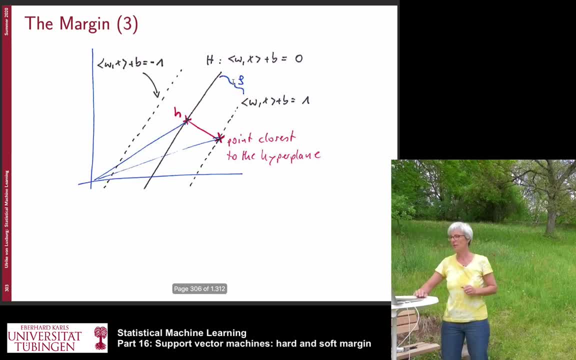 over norm omega. And now maybe I go back to this figure here. The point x is this one here And in vector notation: how can I get from the origin to this point x? I start in the origin, I first move to h. 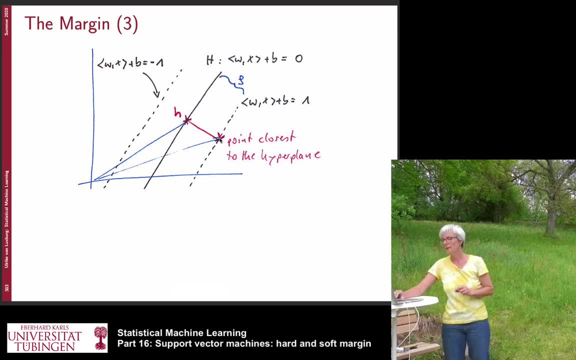 And then I need to move along this red line here. And what is this red line? The direction of this line is omega, that's the normal vector of the hyperplane. And if I want to know how long I need to walk along this line- and we need to take the length- 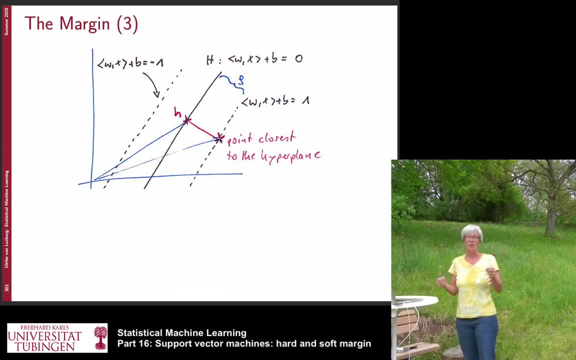 of this line times omega. But now omega might not have norm 1, so I first need to normalize. So if you want to know how long to walk along a certain plane, you can normalize. So now this x equals 1. vector: you need to have a unit vector and then multiply it by the length you want to. 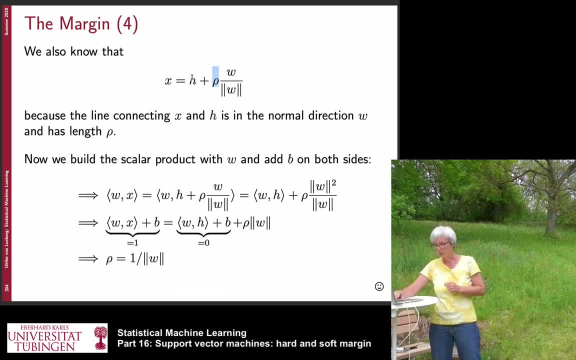 walk. So here we go, from the origin to the point H on the hyperplane, and then, for the length of rho, we walk along this normal vector, w, normalized to 1, such that this equation is true. And now, essentially, we just need to do simple manipulations. Now what we do. 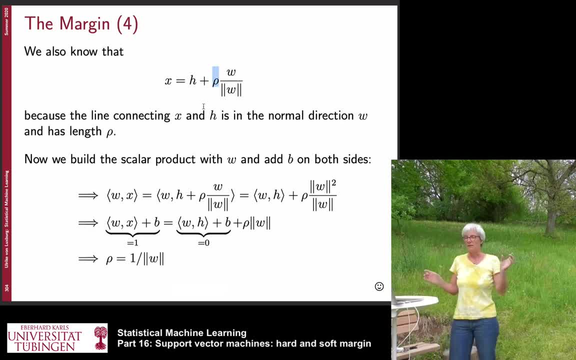 is. this is the equation we start with. Now we take the left side and the right side of this equation and build a scalar product with w. So here we have now w is and w the right side of the equation. So we just took the two parts of the equation and put 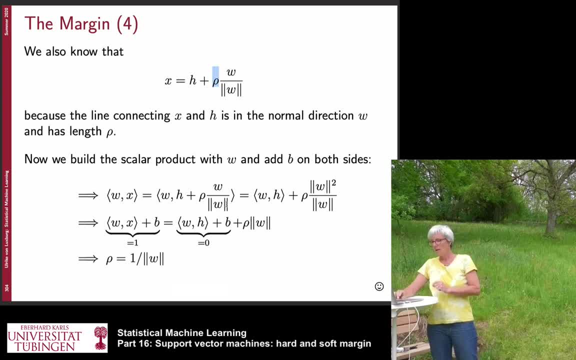 them into a scalar product jointly with w. And now here I can also take out this linear, so it's again a linear form here. so I can put it, pull it into the two parts, And in the next line I can also add b on both sides. If I have an equation, I can add b and nothing. 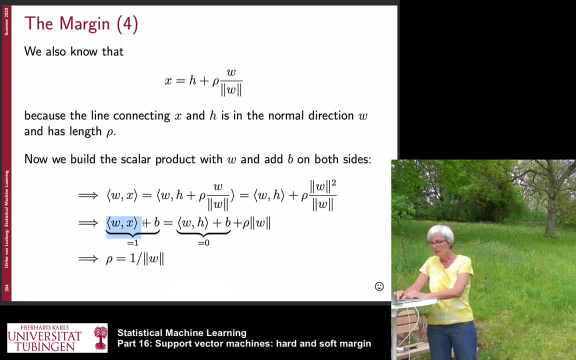 changes. And now you can observe on the left side, we have now omega x plus b, which we know by definition is 1, because this is the way we chose the point. It sits on the margin, so it has to have 1 here because we have canonical form. And here we have omega h plus b, which 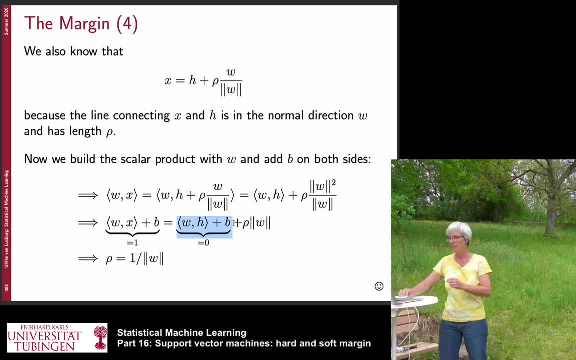 is 0 by definition, because h sits on the hyperplane, And then here's the remaining term. So what we're left with is: 1 equals rho times norm of w, And now if you want to solve for rho, you get: rho is 1 over norm of w, And that's it. That's the part of the 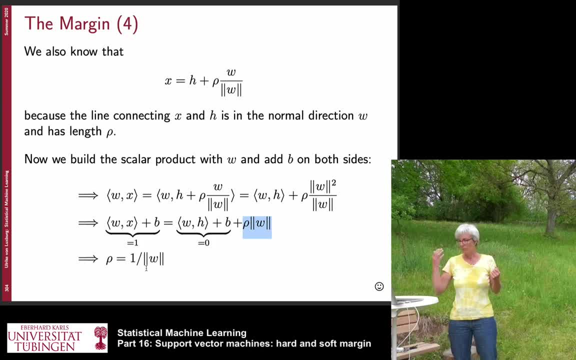 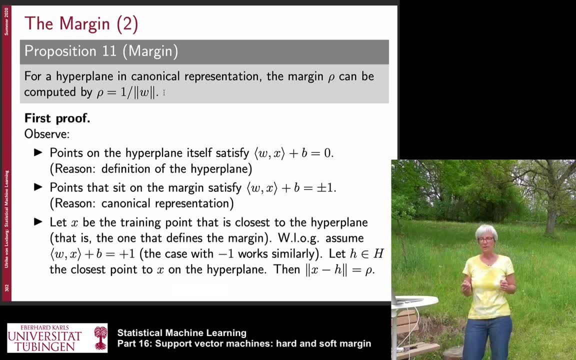 proof, or the easiest proof, for the margin. I go back once more. So what we have proved now is that if our hyperplane has canonical representation, then the margin can be computed as 1 over norm of w. The slides also have an alternative proof. You can read it if you. 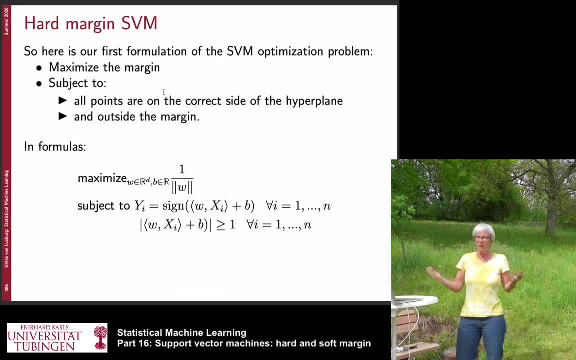 like Now. we already have all the ingredients to define what is the hard margin, SVM. So what we want to do is, given training points and, under the assumption that they are separable by hyperplanes, we want to find a hyperplane that has a margin as large as possible. So 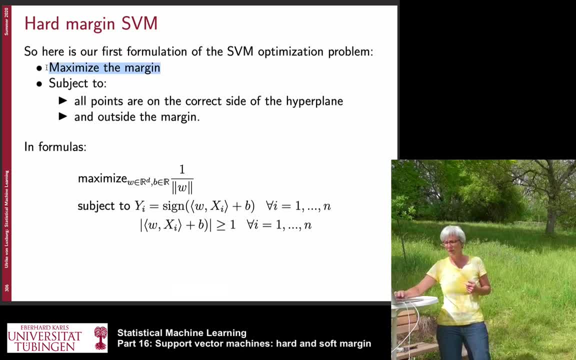 we have an objective function that says maximize the margin, So among all the hyperplanes, maximize the margin. It says in object 2, under the constraints, that all points are on the correct side of the hyperplane and outside the margin. And this sounds a bit funny, so maybe let's. 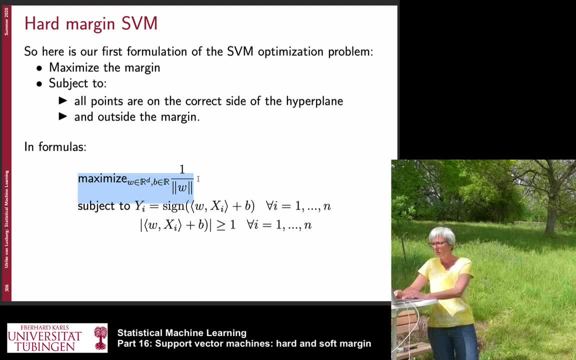 look at it in formulas. So the first one is easy: We want to maximize the margin, so we want to maximize rho, So we want to find a hyperplane, so the parameters w and b, such that rho is as large as possible, which is equivalent to saying 1 over norm of w. So 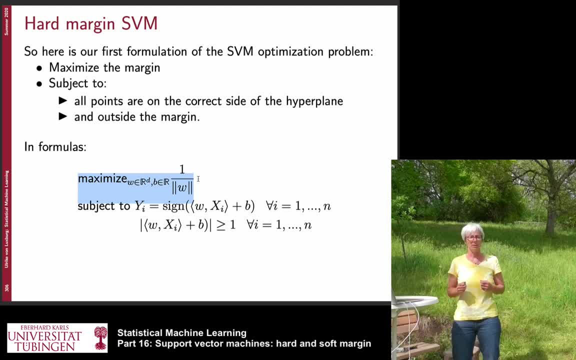 that's an ideal situation. So what we do is that we have to optimize that. So we make a formula 1 over 2.. So it's kind of obvious that we want to maximize rho. We want to find 1 over norm of w should be as large as possible, because rho is 1 over norm of w. 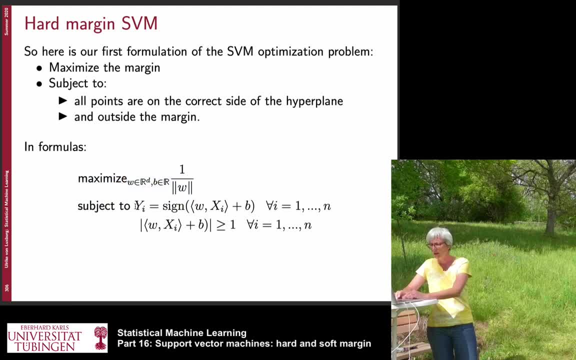 And now the conditions. that's a bit tricky to see. in the first place, What we want is that yi, so xi. yi is a training point. We want that the training point yi equals the sine that the support vector machine gives to that input point. 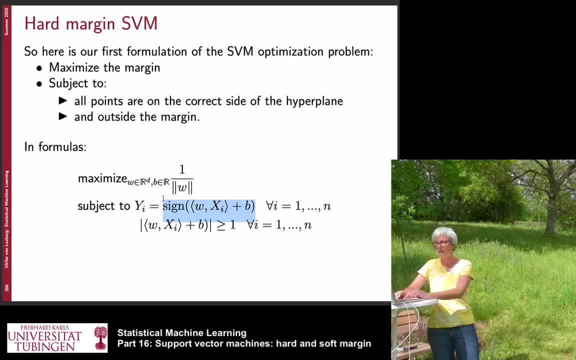 So we put the input, point xi, into our hyperplane equation. look at the sine, and ideally the sine should be the same as the one that's given in our training data yi. This is what we want to have, And then we also want to have that in absolute value, that omega xi plus b is larger or equal. 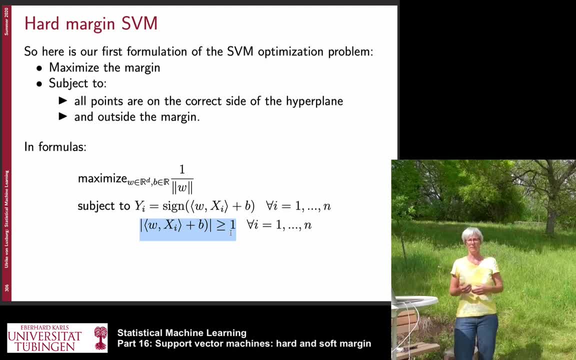 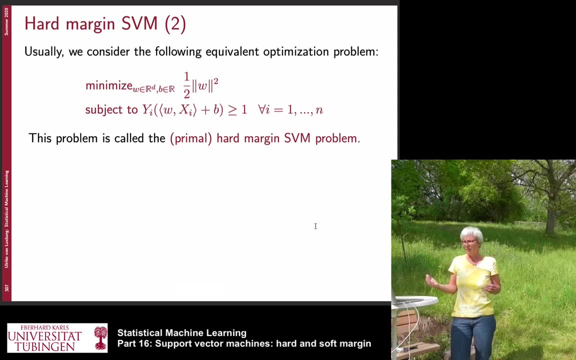 to 1, because we want to have that point sitting outside of the hyperplane, And these conditions we want for all training points i from 1 to n, And typically there is a way to simplify this, To simplify these two things or to change the optimization problem. maybe I go back. 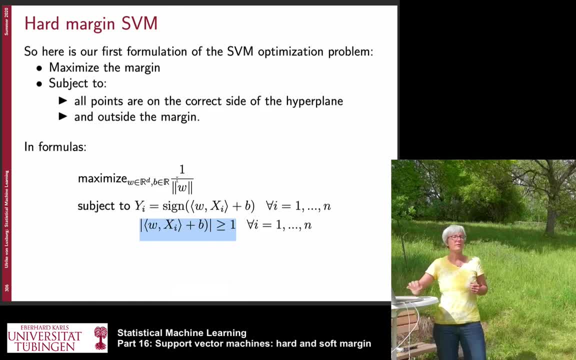 once more. So instead of maximizing 1 over norm of w, which is sort of an inconvenient function for optimization, we could also say we want to minimize the norm of w. So if you take the inverse of an expression, we go from maximizing to minimizing and it's: 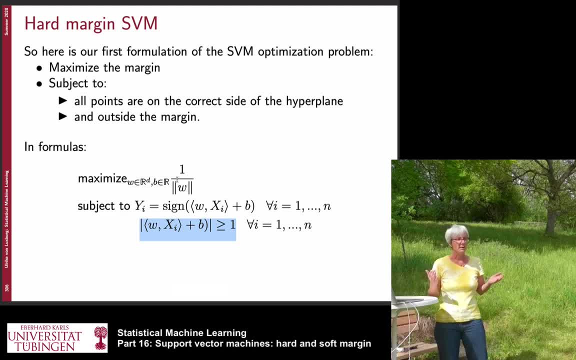 exactly the same kind of problem. Just minimizing a norm is something that's much, much easier conceptually than maximizing 1 over the norm. That's the one change we don't want, Thank you. And now the other change we do is we want to sort of write these cumbersome conditions. 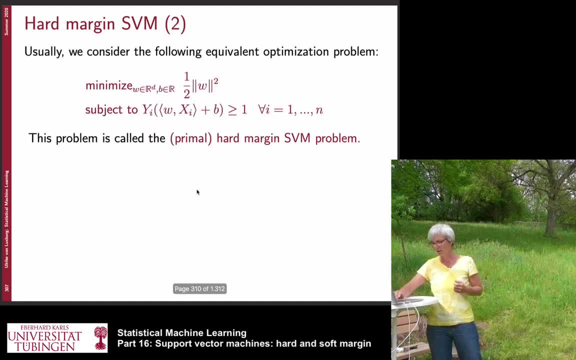 here in a somewhat more elegant way And let's see it on the next slide. So we can subsume both these conditions in one form by saying: we want that the product of yi, the true label, times this expression here, which is essentially the predicted label. 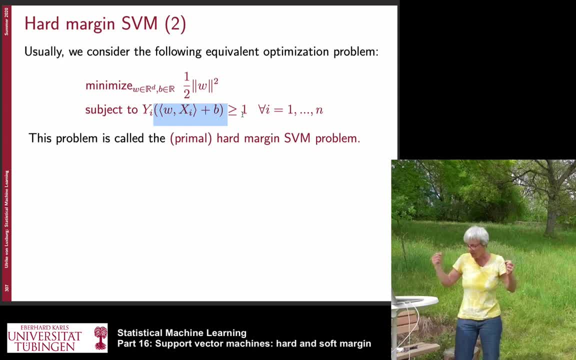 should be larger than 1.. So let's digest this. So this expression here is what the hyperplane spits out for your training. point xi: And the sign of this expression should be the same as yi. So first of all, if you would request that yi times this blue expression is greater, or? 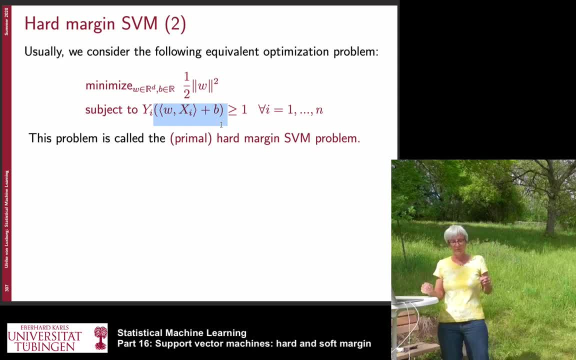 equal to 0, no greater than 0, then we would already request that the predicted sign is the correct one, Because if yi is plus 1 and the predicted sign is plus 1, we have a positive thing here, the same if both are negative. 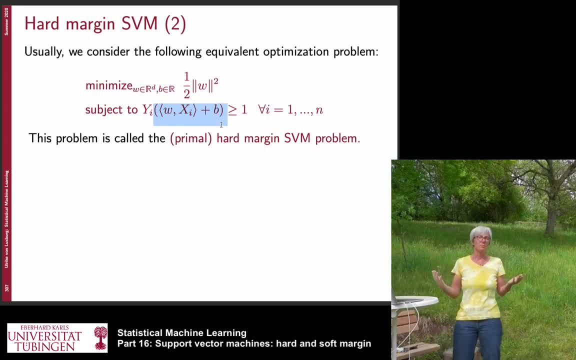 This is sort of In a similar sense, we would request that the predicted sign is the correct one, because if yi is plus 1 and the predicted sign is plus 1, we have a positive thing here, the same if both are negative. 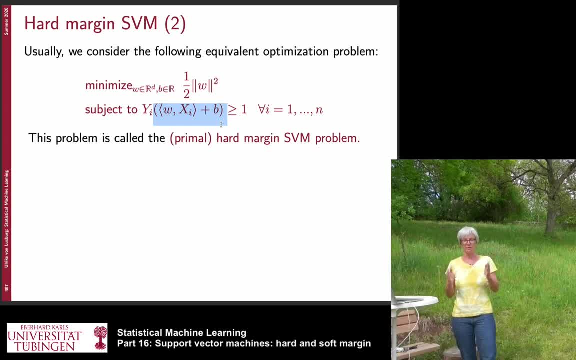 So this is a similar spirit as what we have seen when we looked at the plots for the loss function, So yi times f of x. if this is positive, then we have predicted the correct thing. Looking at it from this point of view, we would say we should have greater than 0 here. 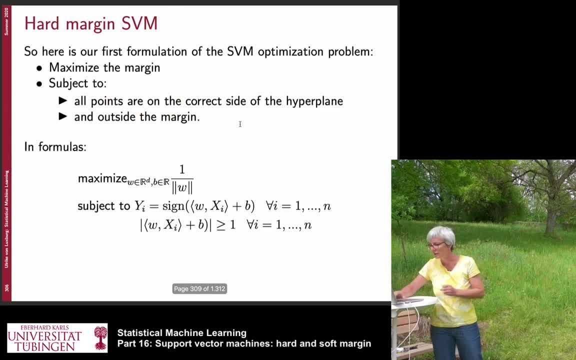 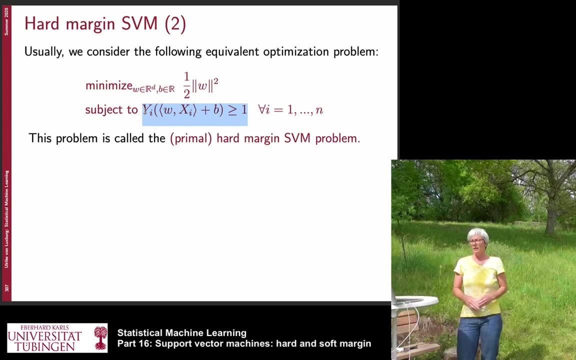 But now we have this other condition. If we go back to the previous slide, we have the second condition, which in fact says it should be larger or equal to 1.. And this is now a simple way On the next slide to satisfy this as well. 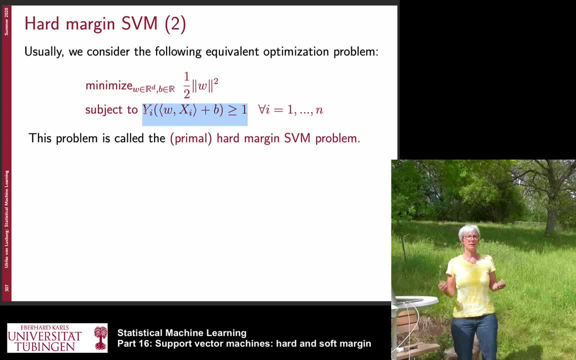 The problem, as it's written here, is called the primal hard margin support vector machine. Maybe one more comment. I added this factor 1 half here in front of the norm of w. This factor 1 half doesn't really change a lot. 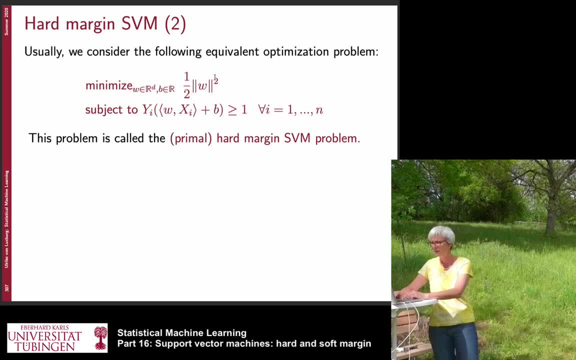 It's just for mathematical convenience. And something else that changed is we added a square here, And this is also for mathematical convenience. Minimizing the norm or minimizing the square of the norm leads to the same solution, But from a mathematical point of view, minimizing a squared function is much nicer. 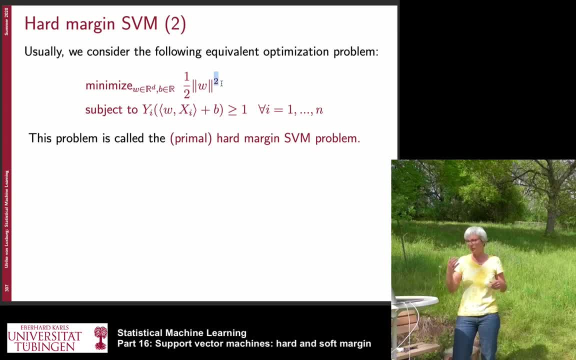 In particular, if you can already imagine what's going on, we might want to take the derivative and then we have 2 times w essentially what is written here, And this is what makes it nicer. So, in the end, this is why people chose this optimization. 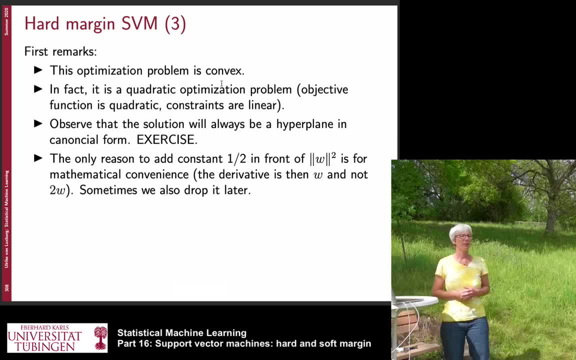 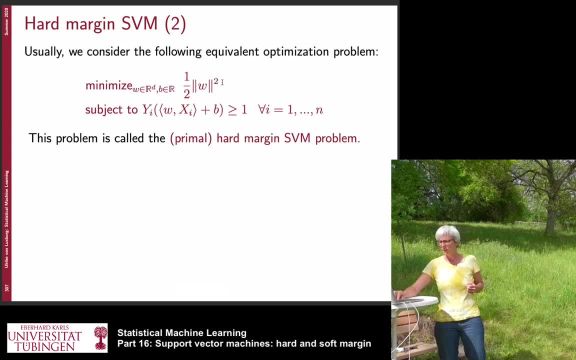 Here are some first insights we could get by looking at this problem. The first one is that it's a convex problem. Let's go back. So the norm here is convex. We have seen that before in the case of regression. So a squared norm is something convex. 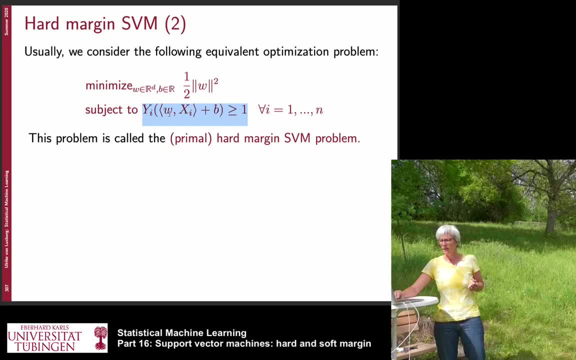 The constraints here are linear constraints. Look again. I mean the coefficients we are talking about is w and b, So it's not so important whether this is linear in x or y, But it's important The coefficients that we want to minimize over in this. x and b, and both occur in a linear. 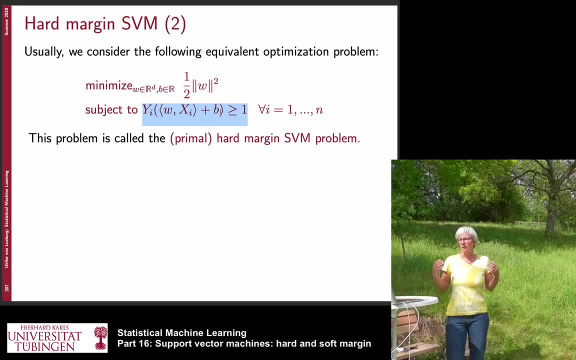 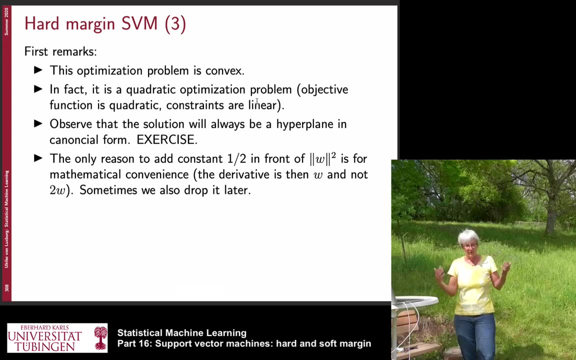 fashion in this expression Now, a problem that has a quadratic objective function and linear constraints. This is called a quadratic optimization problem, And that's a particularly nice optimization problem. This is also what I have here on the next slide, And there are very efficient solvers that are particularly tuned towards quadratic optimization. 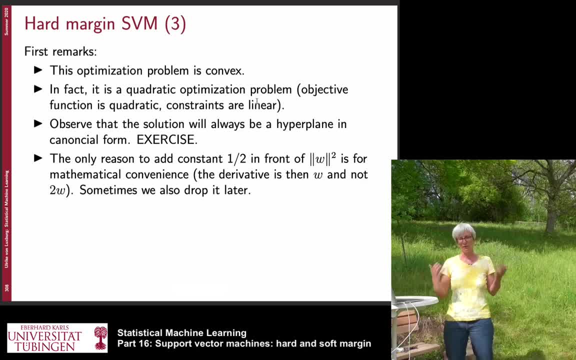 problems. They're convex, but they have a nice structure, So there exist very nice solvers for this one. One thing you might want to observe is that the solution that you find from this optimization problem is always going to be a hyperplane in canonical representation, which is nice. 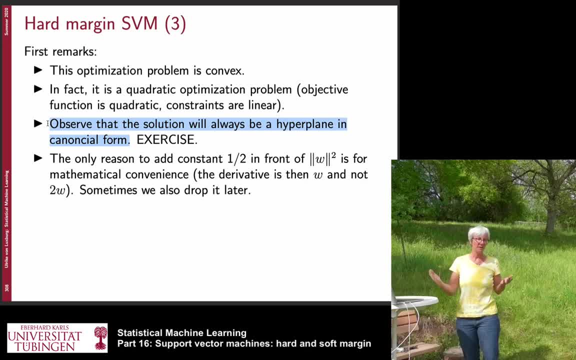 and sort of wouldn't make so much sense if it wouldn't be the case. But this is still something that's not obvious. So you might want to prove that. We might put it on an exercise sheet. If we don't, you might want to prove it anyways at home. 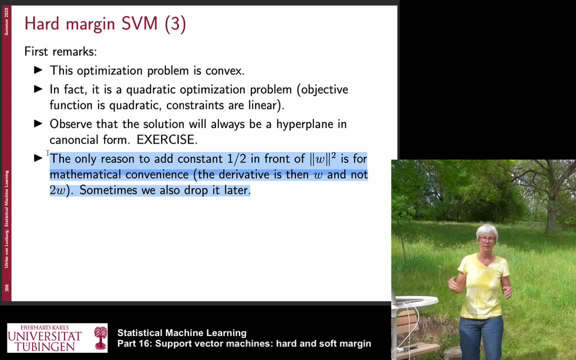 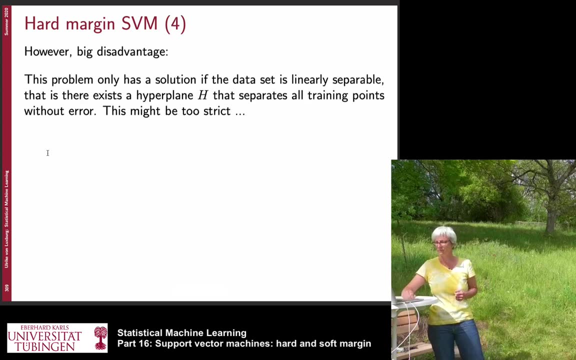 And here I wrote again that this reason to have the constant one-half is sort of the mathematical convenience, And we are often very sloppy with constants, I wrote here. sometimes we even drop it later because we don't want to take track of all the constants in the optimization problem. 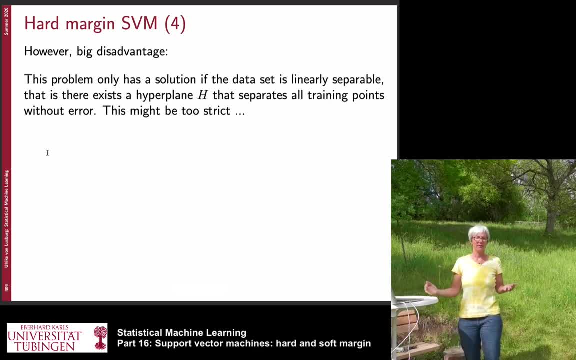 Now this is all nice, but there's obviously a very big disadvantage, which is that currently we always derive the support vector machine just for the case where the two classes are separable. So if there exists a hyperplane that really separates the two classes, 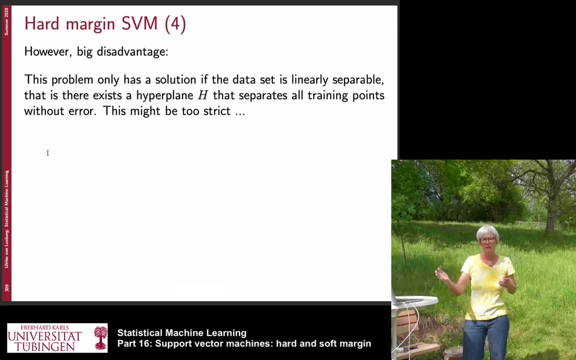 If there doesn't exist such a hyperplane, this thing breaks down, because the definition of the margin doesn't really work anymore, because it always assumes that we can separate the data points And if we cannot, then sort of we need to think about what to do instead. 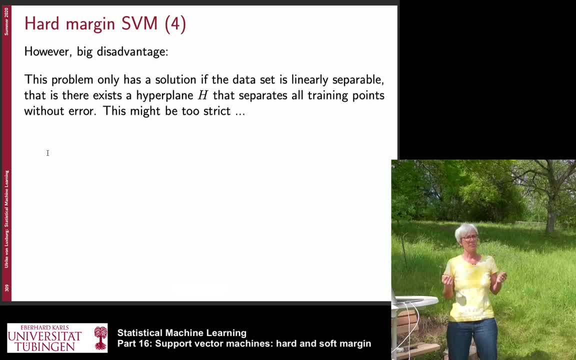 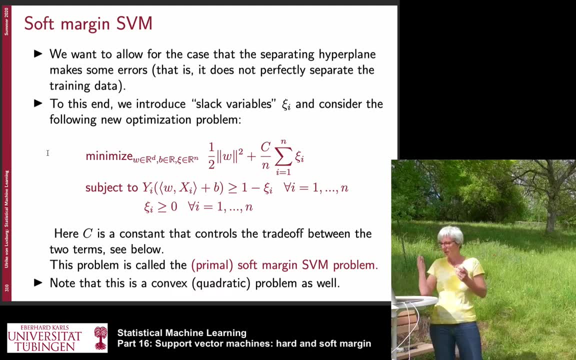 So what we are going to do, then, is to derive what is called the soft-margin support vector machine, which is going to solve this problem. This comes on the next slide. We now want to allow for the case that the hyperplane is not going to have the constant. 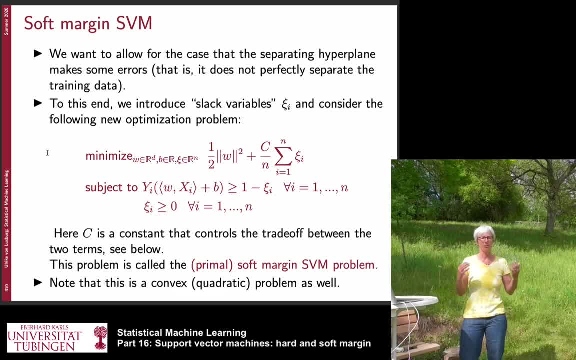 hyperplane can make some errors, So there might be some training points which are ambiguous, which might even belong to a wrong class. It might also be that the problem is not separable at all, like in the example where we wanted to classify people as being female or male. 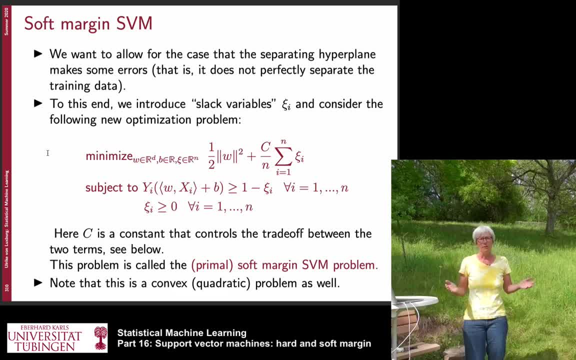 based on their height of their body, And, of course, there is not a unique solution that always predicts the correct thing. So, no matter how we would put a classifier here, there would always be some people who were mispredicted, And this is the case we now want to treat. 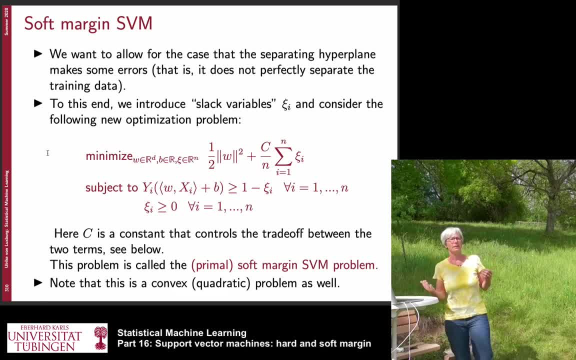 Now, in optimization there is something very common that we try to do. We say, okay, here is a condition, the hard margin condition- that I cannot always satisfy. What I am going to do is allow for not satisfying this condition, but I measure by how far, essentially, I violate. 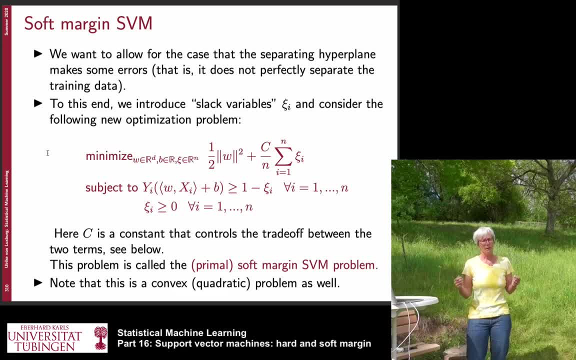 this condition and then I punish. The more I violate the condition, the more I punish, and I'm trying to prefer solutions where this punishment is small. Now let's look at it in this particular example. What we now do is we introduce what is called a slack variable xi i. So for each data point x- i, we introduce a. 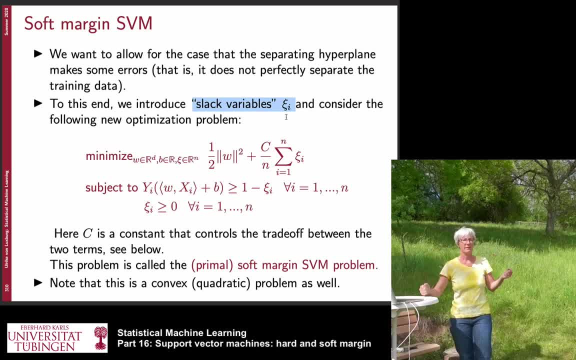 slack variable xi, i, and essentially the slack variable is supposed to measure how far this particular data point sits on the wrong side of the hyperplane, if it does. So what we're going to do is we look at an optimization problem. the objective function now gets extended- the first part here and this one half norm. 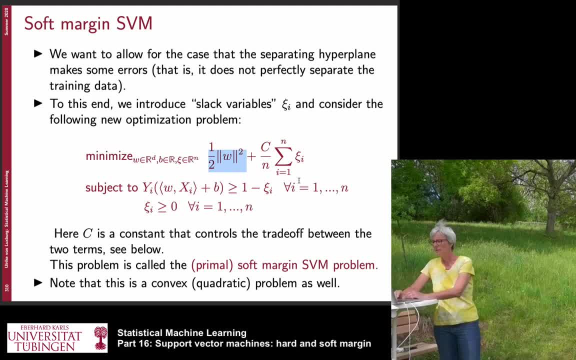 of w squared is still the same as we had before, but now we have a second term which, for some funny reason, I cannot mark with my mouse pointer. but don't worry. So c over n is just a trade-off constant. we are going to discuss it. 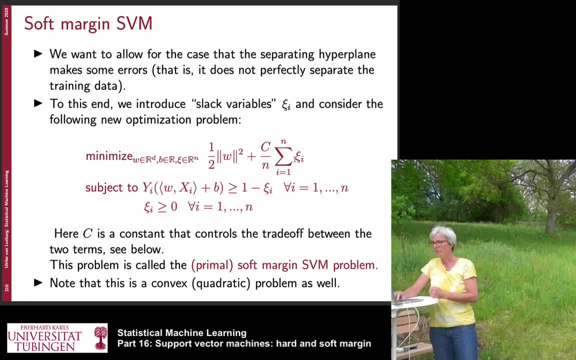 later. but what is important now is this sum over xi i. So for each data point, this xi i is supposed to be something like this: So this is the sum over xi i. So for each data point, this xi i is supposed to be some kind of punishment term and we sum over all these punishments and then the 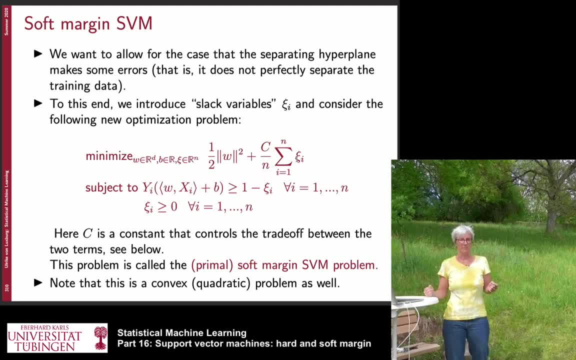 sum of all these expressions should be as small as possible. So we have two different ingredients here. We have that the margin is supposed to be small and the punishments are supposed to be small at the same time. But now, how do these punishments work? This is sort of hidden in the constraints now. So previously, if 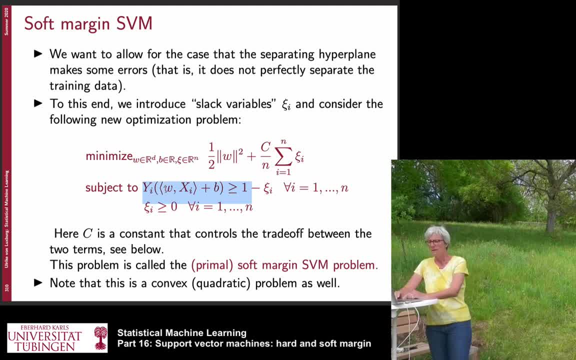 you remember, we had the constraints and yi times w, xi plus b is supposed to be larger than xi i. So what we're going to do now is we're going to take the constraints and yi times w xi plus b is supposed to be larger than one. This was the hard margin. 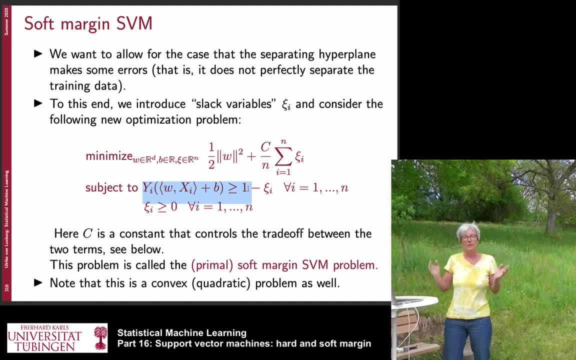 constraint. Now we allow that the thing is not larger than one. It can be something smaller, So the expression here can be smaller than one. now Xi i is going to be a positive number. We have that here. So all xi i's these. 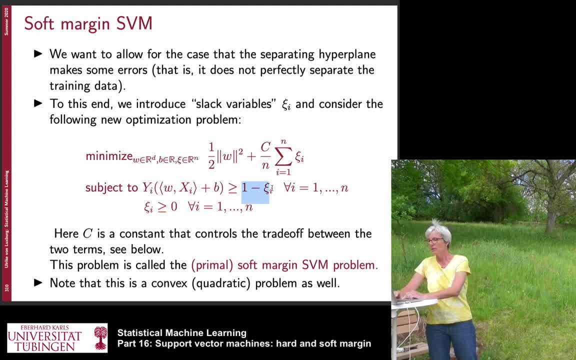 punishment constants are positive or non-negative. So when say xi i is 0.5, then we have here all of a sudden we don't have its larger equal to 1, but only to 1 minus 0.5, so 0.5.. 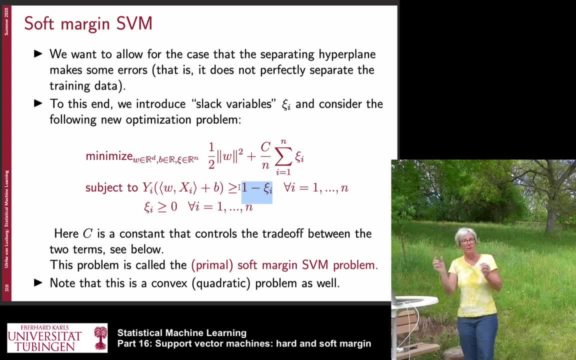 But now this 0.5 sort of, by which we just by which we go beyond the 1, this is going to end up in our punishment term. So this 0.5 here is now in the sum which I cannot mark with my mouse pointer. 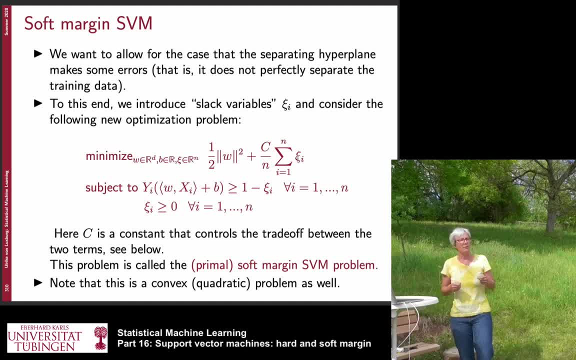 And now there's like: if I have a data point, there are two cases. It could be that it's very easy for this data point to be on the right side of the hyperplane and then I don't have any punishment term. Then I simply choose xi, i is 0 and I'm on. 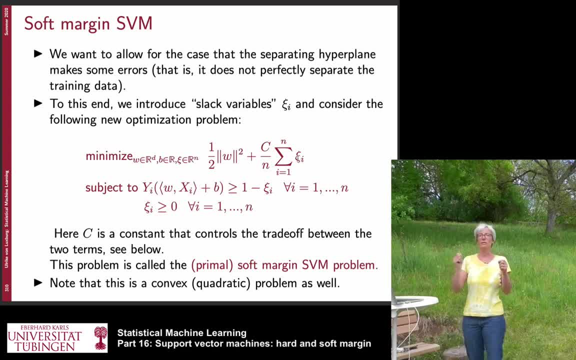 the right side of the hyperplane, as I would have been before. But now, if there's a certain point that would sit on the wrong side of the hyperplane, I'm still allowed to choose that hyperplane, But I incur a punishment that depends on how much this. 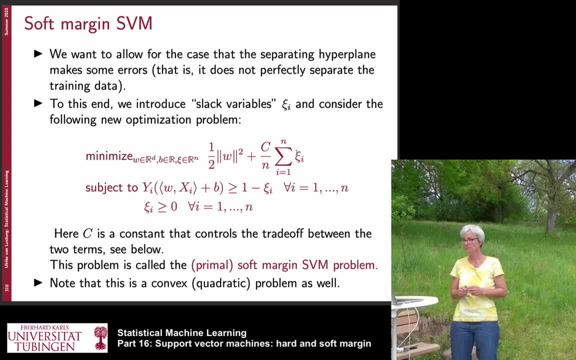 point sits on the wrong side of the hyperplane, So this is sort of a standard approach that is taken very often in optimization. If you cannot satisfy a condition, then introduce this kind of slack variables and try to minimize the violations of this condition. The constant c here. 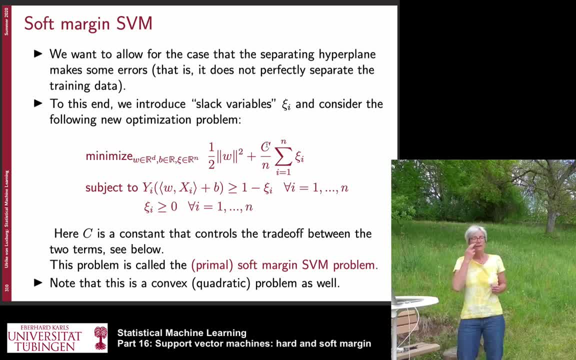 that we have in front of this violation term. it's called the c parameter of the support vector machine. It's always called c in the literature. This is a kind of trade-off constant, as we had in ridge regression or so, which controls the trade-off. 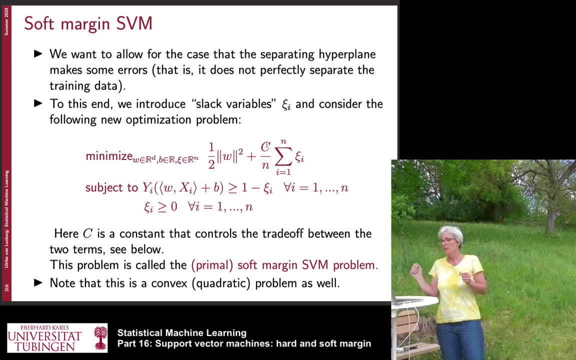 between the two parts. Again, there might be different weights. so if you choose a very large c, then it's very important to us that we do not have points on the wrong side of the hyperplane, Because if c is large, then this term here is supposed to be 0.5.. So that's a little bit of a. 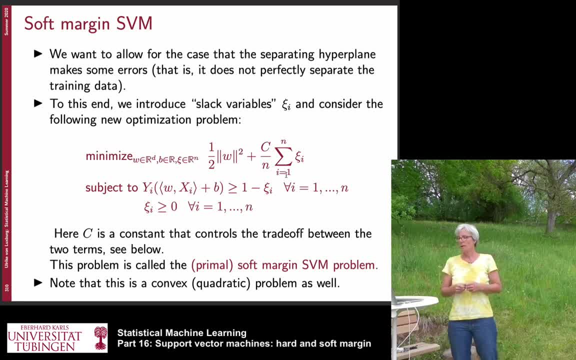 challenge for us to become very small. And if c is very small then we say we don't even care about this punishment. hopefully the margin is going to be small And this is called the soft margin support vector machine, because if now this margin condition has been softened and this is why it's called soft margins SVM. 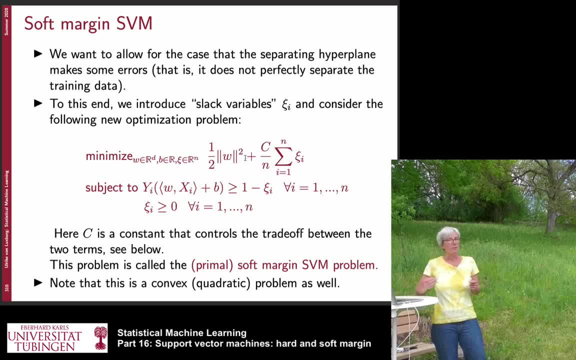 Note that this problem is also a quadratic optimization problem, Because the objective function is still a quadratic function. now maybe consider what are the variables that we have in our optimization problem. We have the original variables w and b, but we now have n, more variables. 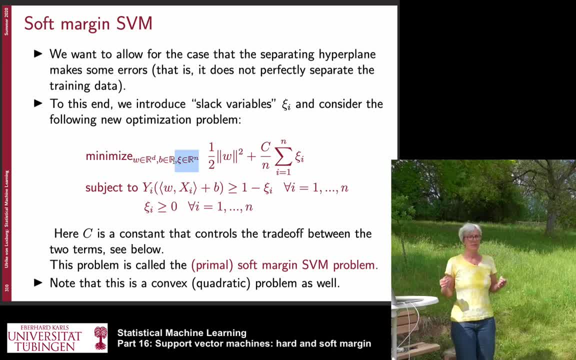 All these lag variables are also variables that we need to optimize. So not only do we now need to find the parameters omega and b, but at the same time, also these parameters xi, i, And this is still a function that is quadratic- in all of these ingredients. 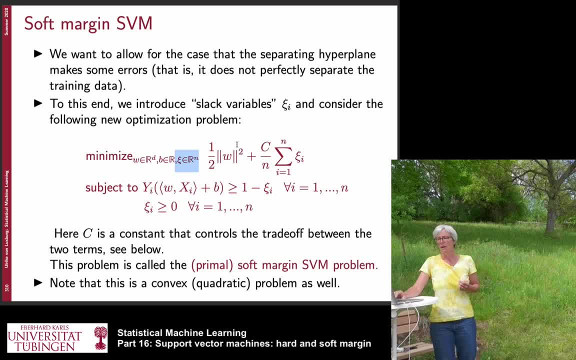 So this term is quadratic in omega, this is linear in the xi's, and something that is a sum of linear and quadratic terms is still a quadratic function. So the objective function is still a quadratic function, a bit more complex than we had before. 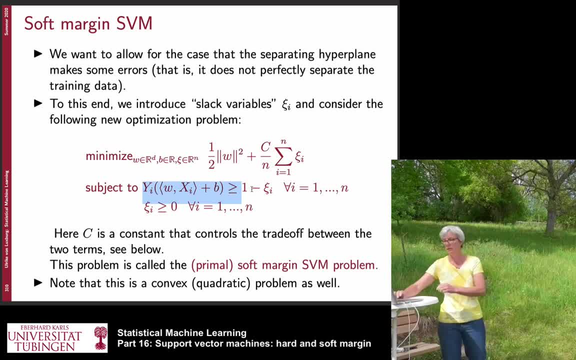 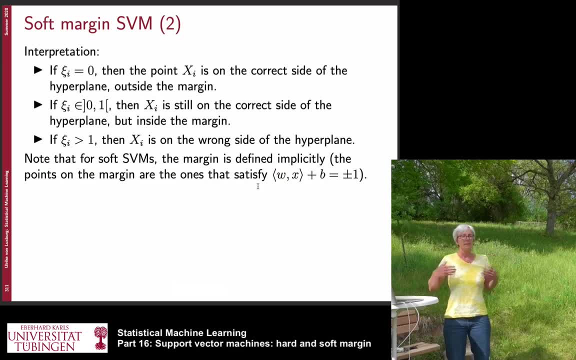 but still- And this is still a linear function, it's more or less the same. This is also something that's linear in xi i. Now there's a geometric interpretation to these parameters xi i, to these punishment parameters, and I want to show you this interpretation. 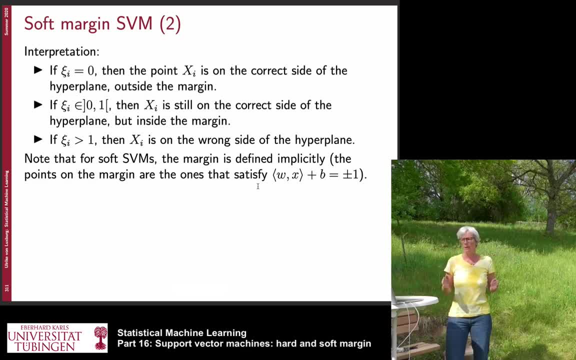 The first one is: if xi, i is zero, then the point is on the correct side of the hyperplane and it's even going to be outside of the margin. Because what we say is: and we want to have, like in the hard margin case, we want to have 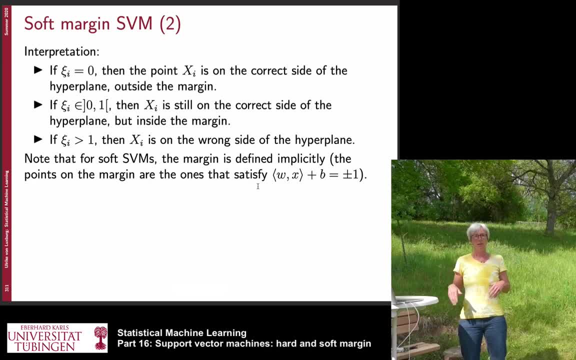 all training points outside of the margin on the correct side, If we do not punish. this is exactly the case Now. what we're going to see on the next slide is if xi i is in the interval between zero and one, then xi i is still going to be on the right, on the correct side. 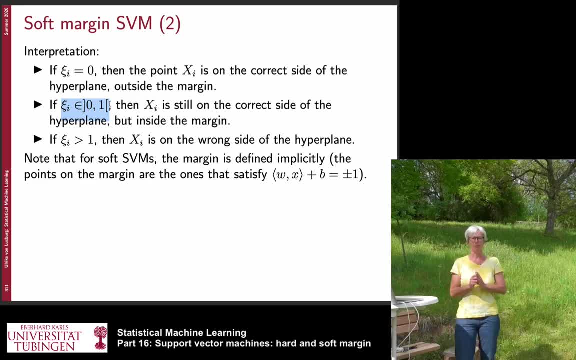 If xi i is in the interval between zero and one, then xi i is still going to be on the correct side of the hyperplane but already has moved into the margin. And if xi i gets larger than one, then the point is even on the wrong side of the hyperplane. 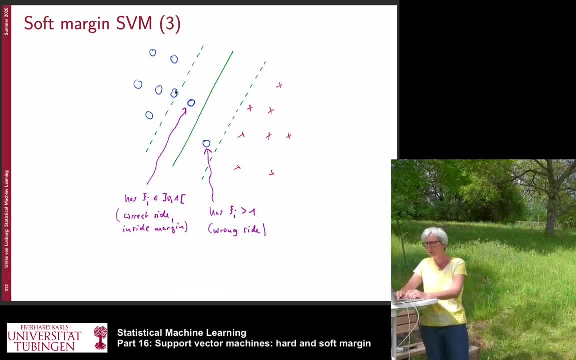 Now maybe let's look at a figure that's easier to see. So here we have a couple of points: The blue circles are one class and the red crosses are the other class. We have a hyperplane here And the dashed lines indicate the margin. 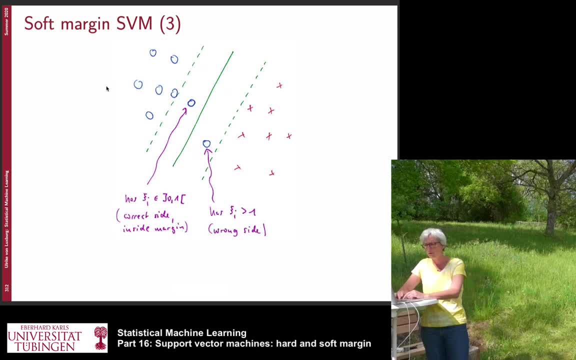 So, for example, this point here- Well, I can't mark it, sorry. This point here sits outside of the margin on the correct side, so it would have xi. i equals to zero. There's no punishment at all for this particular point. 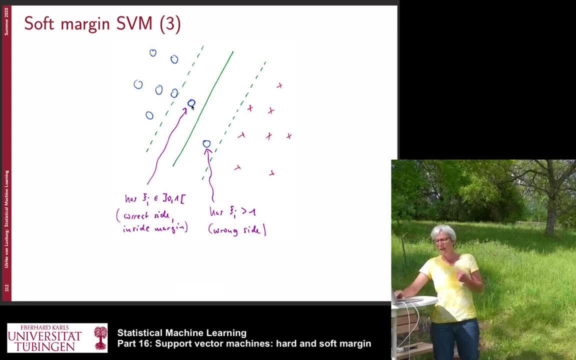 Now this point here, which has this arrow pointing towards it, that already sits inside the margin. It is still on the correct side of the hyperplane, but it's inside the margin And we would like to have the points not inside the margin because we want to have a large. 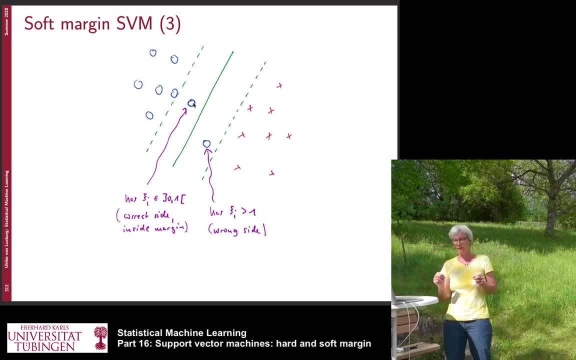 margin. So we are going to punish this point. This is some parameter xi i Which is between zero and one. And then this point here: this circle, for some reason, is on the wrong side of the hyperplane And this gets punished even more. 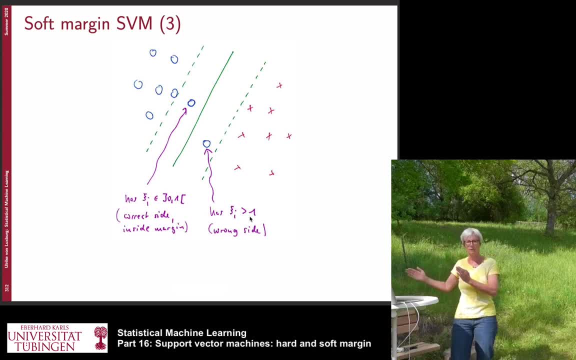 And it has a xi i that is larger than one, And the more it's going to be on the wrong side of the hyperplane, the more this xi i is going to grow and the more it's going to be punished. So if this point is somewhere very far outside, beyond the red crosses, the punishment is 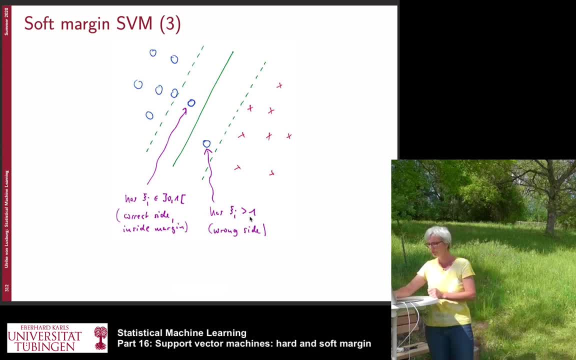 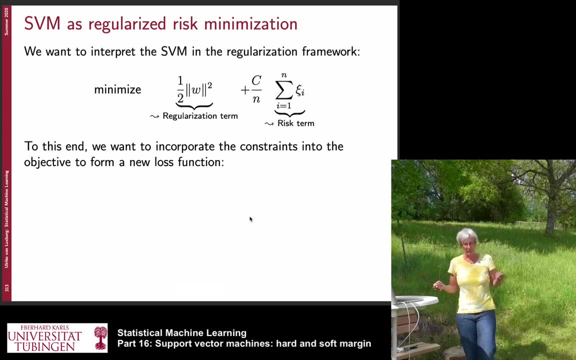 going to be enormous. And with this intuition, we can also now understand the soft margin, SVM, in terms of regularized risk minimization. If you maybe forget about the constraints for the moment, just look at the objective function. We have one term which says minimize the margin or maximize the margin. in terms of minimizing, 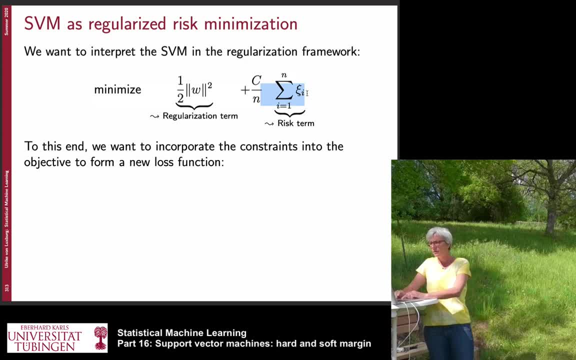 the norm of w squared. And then we have this term here, which we can now interpret as some kind of risk term or loss function. So, And what we want to do is we now want to find the loss function such that this sum of xi. 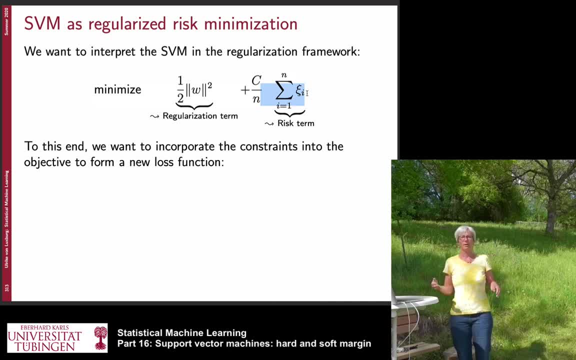 i- is in fact the loss of the classifier for these particular data points, And then the first term here this is going to turn out to be the regularization term. As you can see, it does not directly depend on individual training points. It's more like a property of this function. 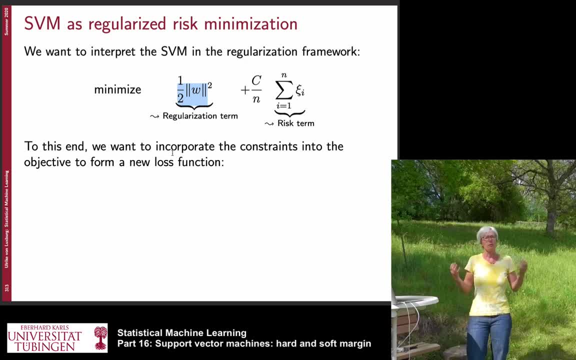 And as we used to regularize in rich regression, for example by the norm of w or this, like depending on, in rich regression we use the square norm, We might also punish by the L1 norm, And this is sort of a similar spirit. 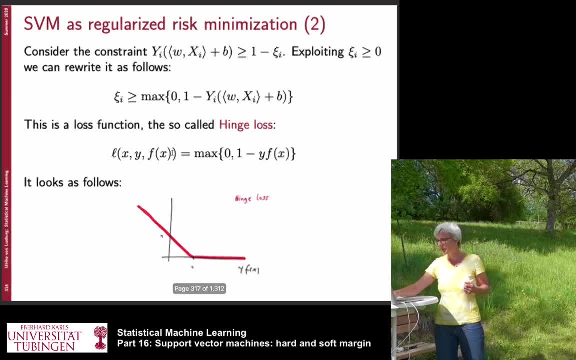 So this would be the regularization term And let's maybe go towards the place where we can try to prove what is this loss function And to see this. what we're going to do is we take this linear constraint that we have that involves these xi- i parameters. 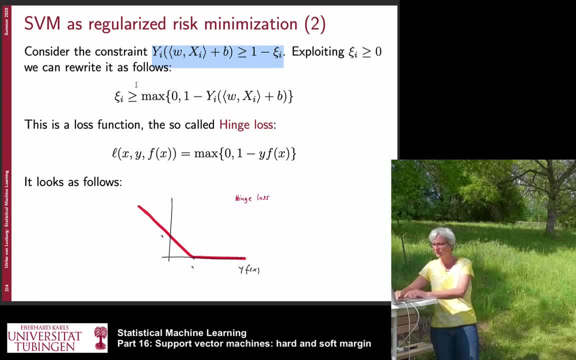 And this can be easily rewritten. you need to be a bit of trickling by saying xi: i is larger or equal than the maximum of either 0 or 1 minus yi, omega xi plus b. Okay, so there might be two cases. 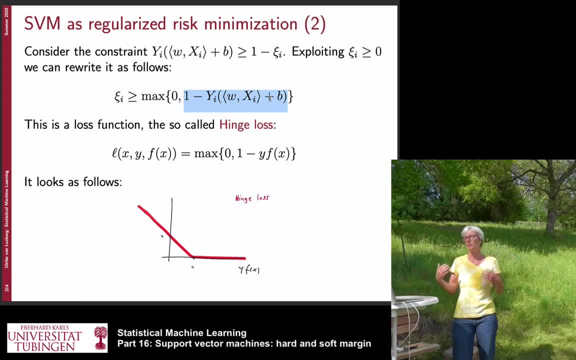 Either the point is classified correctly, then we don't incur any loss. xi, i is 0 and we're happy. And you can see that if a point is classified correctly, then this expression here is larger or equal to 1.. Sorry, if a point is classified correctly, this expression is larger or equal to 0. 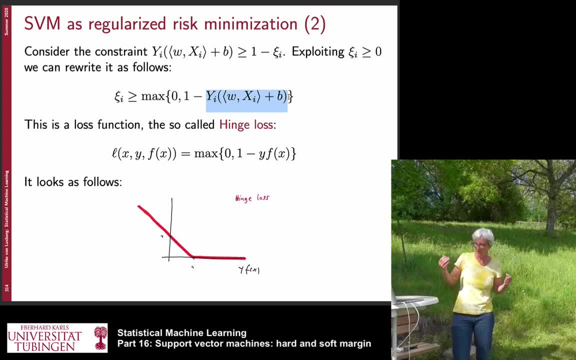 Ah, okay, exactly, We need to, and here we come. if what I said was not entirely correct, If a point is classified correctly and is outside of the margin, it doesn't incur any loss. So if this term here omega xi plus b, if the absolute value of this term is larger, 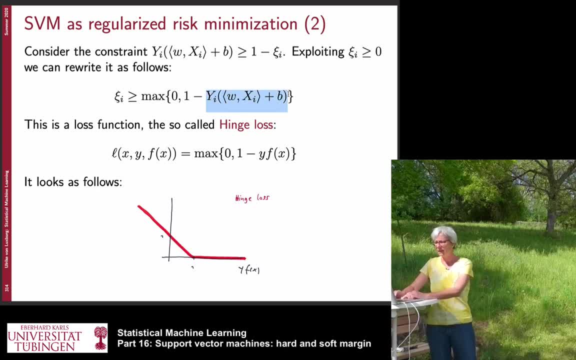 than 1, and it has the same sign as yi. This means that the training point xi is classified on the correct side and sits outside of the margin. And then this expression: here we have 1 minus something that is at least 1.. 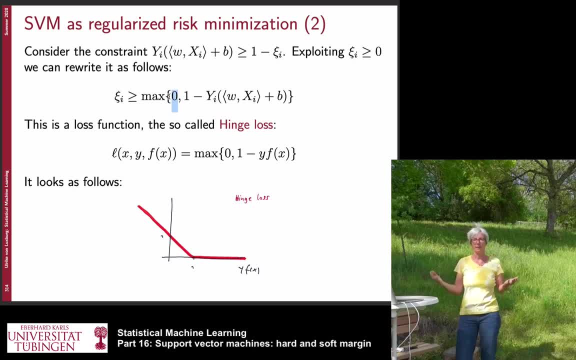 So we are left with the maximum, which is 0.. So the xi i is 0, we don't get any punishment. If we have a point that is on the right side of the hyperplane but maybe it's inside the margin, we start incurring a loss. 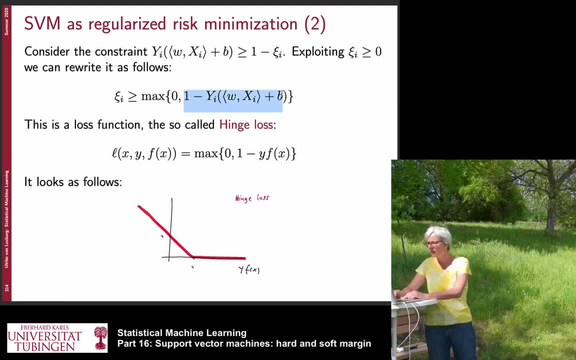 And essentially this number here measures, or this whole number here measures, how far we are inside the margin. If we sit right on the margin, this term yi, omega xi plus b, is exactly 1, so we don't have any loss. But as soon as we start moving in the margin, we have a loss that increases linearly according. 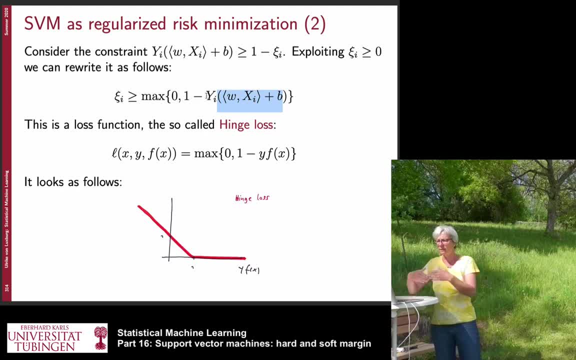 to how far we are from the margin, And if a point now sits on the wrong side of the hyperplane, it increases even further. So then this expression here becomes something that is negative, And we have minus, something negative, so it's positive. so this gets even a larger number. 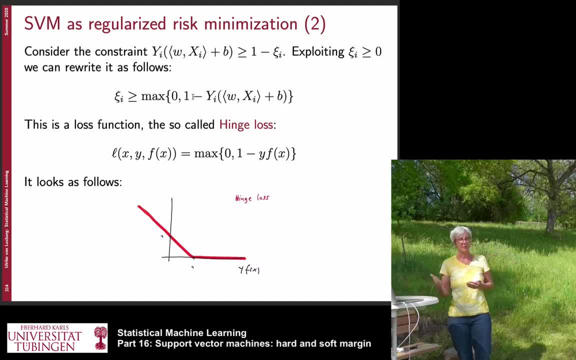 And now we can define- essentially we can define- a loss function by this expression. What we now do is we simply define a loss for input data x and y and the predicted value f of x, And the loss is defined exactly as the expression we had before: the maximum over 0 and 1 minus. 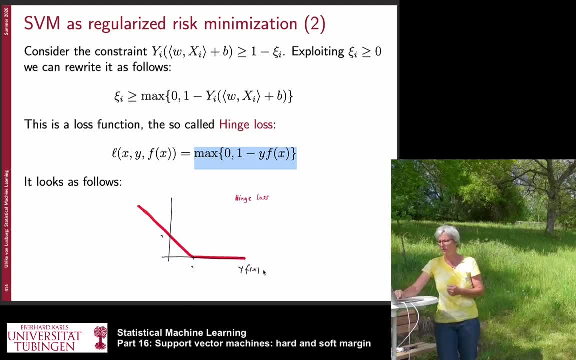 y f of xi, And if you plot this, you get the following expression: If you plot this loss, it looks exactly like this one here. So on the x-axis, we have again, as we have seen it previously, yi times f of x. 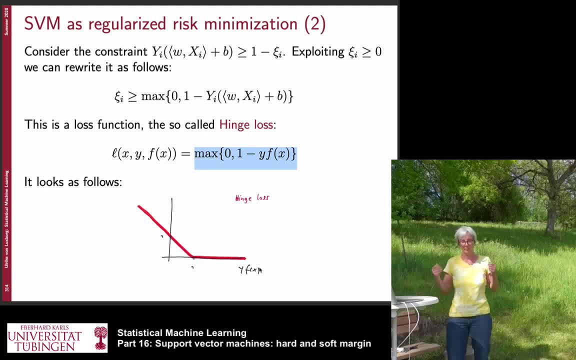 So we have again: if yi times f of x is positive, then we classified the point on the correct side. If it's negative, it's misclassified. But we can see now the loss. already not only the loss starts to count if we are on the 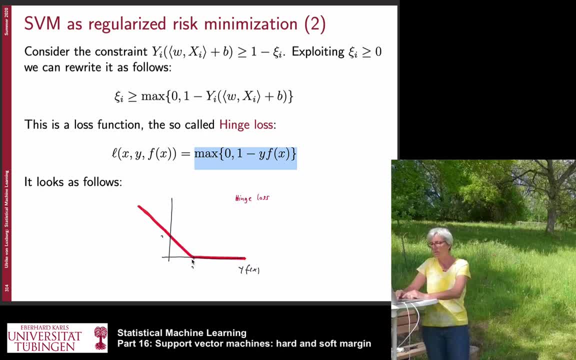 wrong side of the hyperplane, but it already starts to count if this expression gets smaller than 1.. These are the points for which we have a loss. These are the points for which we sit inside the hyperplane, but on the correct side of. 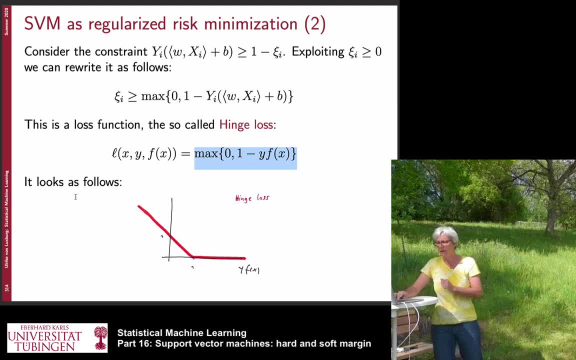 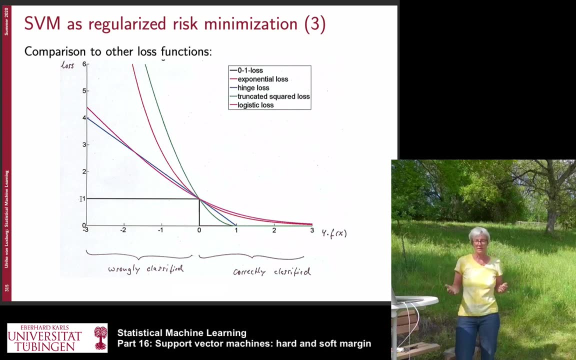 the margin And then, once we move beyond the zero line, here we are on the wrong side of the hyperplane and the loss increases linearly depending on how far we are away from this hyperplane. I also want to show this loss function in the context of other loss functions. 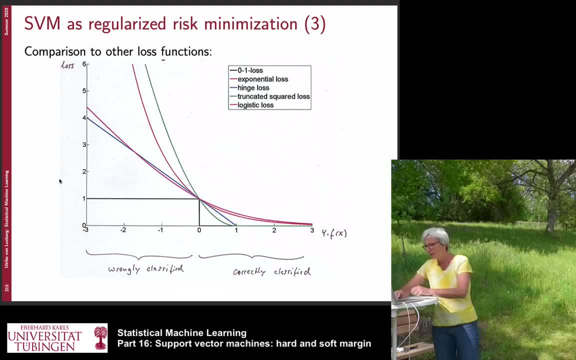 And we have seen this plot already before. Now let's see the hinge loss. It's this one here. As you can see, it increases linearly If we go out, if we go to the wrong side, And this is essentially very close to what the logistic loss does. 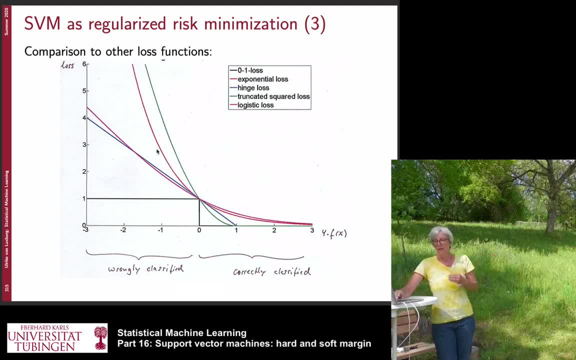 The logistic loss also more or less increases linearly, Whereas many of the other losses, like exponential loss or squared loss or so, they increase in a much, much more faster way. when we go to the wrong side of the hyperplane- And it is sort of a robustness kind of feature of SVMs and also logistic regression that the loss only increases linearly. 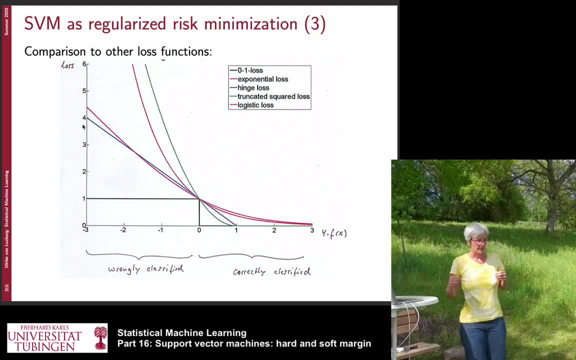 Because somehow, if you have a point that by all means you cannot classify correctly, and, for example, you have an outlier at a point and it sits far away from everything else, If the loss grows quadratically with the distance of this point to your classification or to 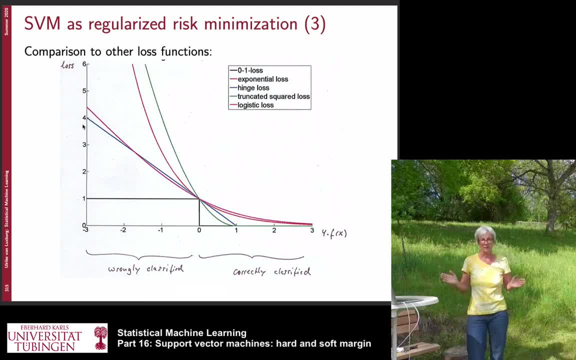 the other points, then essentially this point is going to dominate everything, And this you don't want So often in robust statistics. what we do is we try to only punish in a linear fashion, And this is what happens in the hinge loss here. 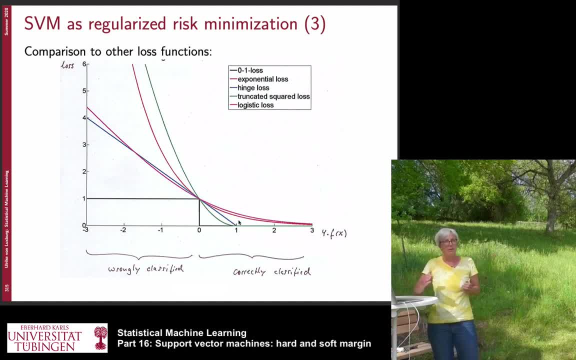 And, as in the case of the logistic loss, we only punish in a linear fashion. And this is what happens in the hinge loss. here, And as in the case of the logistic loss, we only punish in a linear fashion And logistic loss as well, we still have punishment if we're on the correct side of. 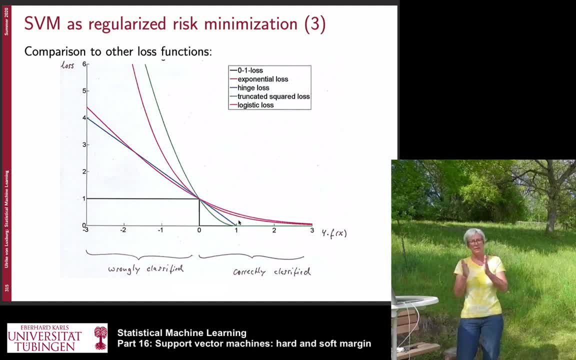 the hyperplane, but only as long as we are inside the margin, And as soon as we're outside of the margin we do not have any particular loss anymore. So then we incur zero loss, Whereas the logistic loss, for example, it's this red line here. 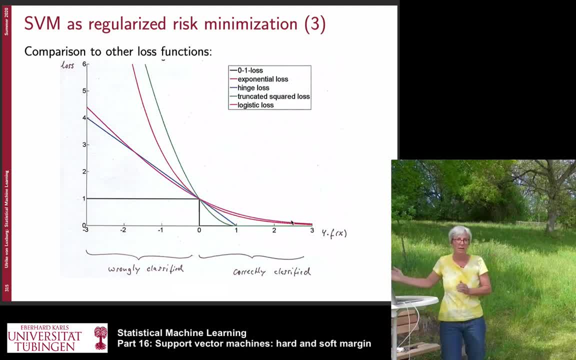 It still incurs any loss. The loss goes to zero and at some point gets negligible. You can sort of ignore it, Whereas for the support vector machine we stop at some point to encounter any loss as soon as we're essentially on the right side of the margin and on the right side of the. 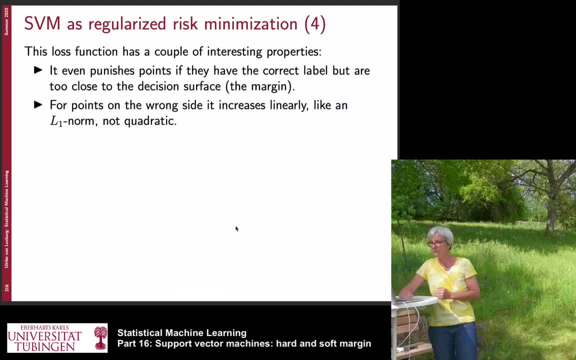 hyperplane. Okay, here again I summarized the properties of this loss function, but I think I mentioned all of them already. So the loss function punishes points, even if they're still on the correct side of the hyperplane, but inside the margin. 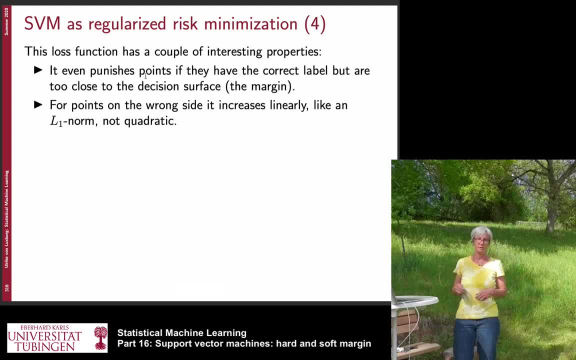 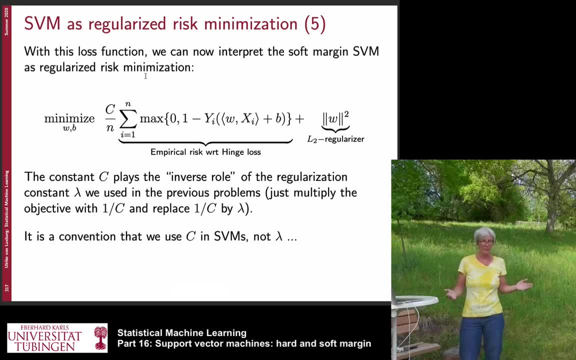 And it increases linearly, not quadratically or in any other way. So this is the loss function Now. it's not going to change in any other way once we go on the wrong side of the hyperplane. So now we have this loss function and now we can in fact interpret the soft margin, SVM. 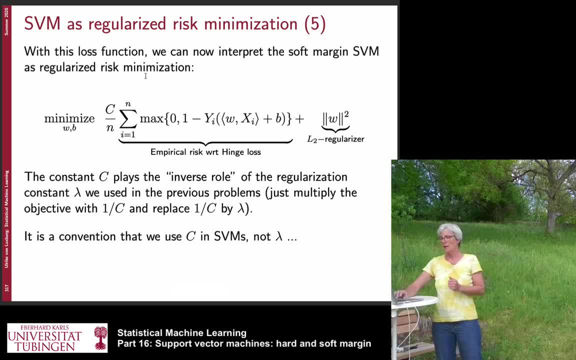 in a standard regularization kind of framework. Our problem now looks as follows. I simply rewrite. It's exactly the same kind of function we had before. It's just arranged in a different way because in empirical risk minimization or in regularized risk minimization. 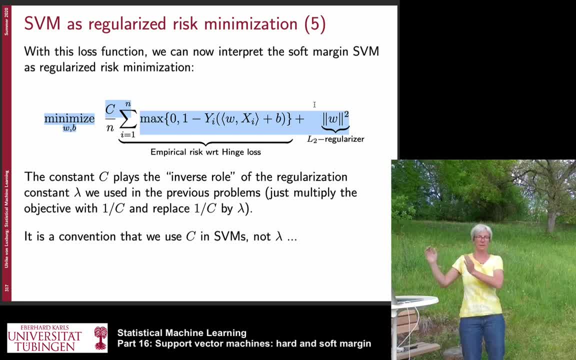 The standard form is minimized, It's just in a different way: minimize regularized risk plus regularization term. no, sorry, minimize empirical risk plus regularization term. so i now change the order to have the same kind of thing. so here is: minimize the empirical risk with respect to the hinge loss. 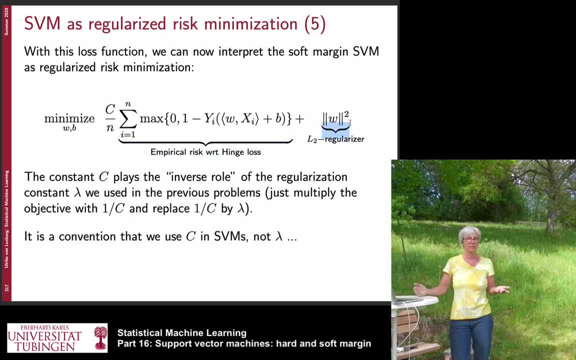 plus the regularization term. as i said before, essentially what we have here is a squared norm regularizer and the only difference- but that's sort of for historic reasons and between this expression and the one we had, for example, in in rich regression, is that the trade-off constant. 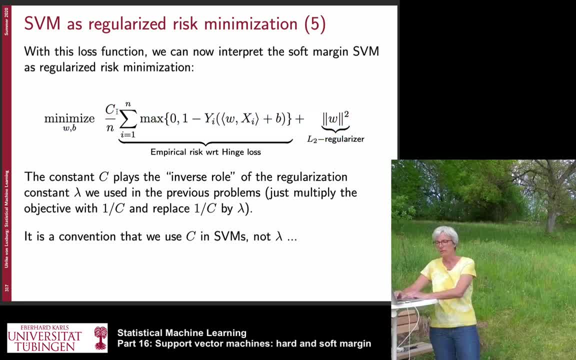 for support vector machines is in front of, in front of the risk and not in front of the regularizer. this doesn't really matter. you can observe sort of the same kind of behavior. you can now think about what happens if c is small and what happens if um, if he gets large, and it's sort of inverse. 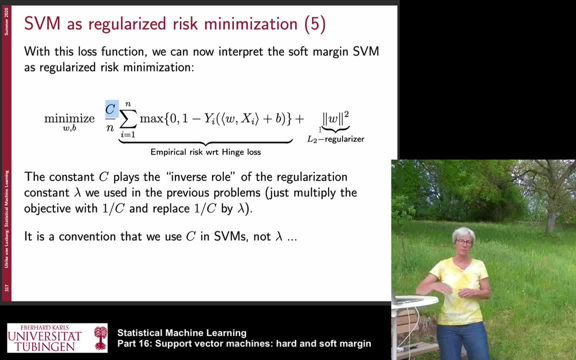 to what would happen if we would have a constant here, lambda, and this lambda is going to be small and large- you can maybe try to figure it out yourself- and it's simply a convention. This is because the first couple of papers for support vector machines started to call this constant C and put it in front of this risk term, and it simply 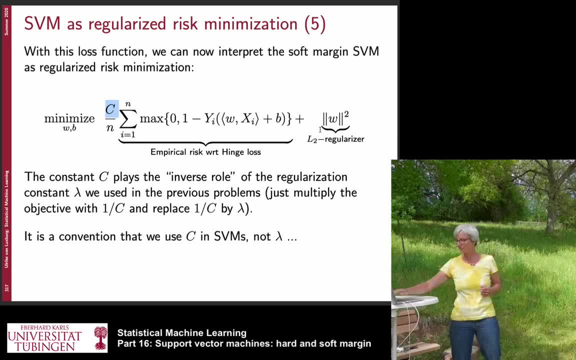 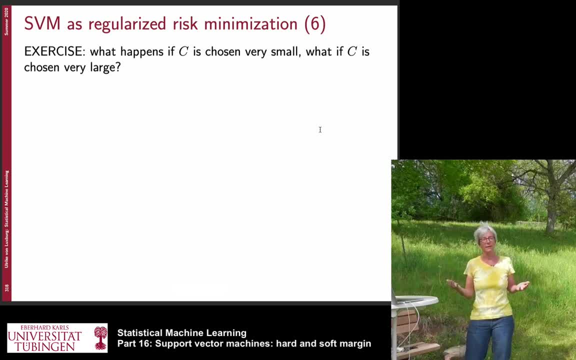 stayed this way in the literature. Okay, I already mentioned it, but you might want to take it as an exercise. If you drive C very large, what is going to happen? And if you drive C very small, what is going to happen? What are sort of these boundary cases of SVMs? In which ones do we underfit in? 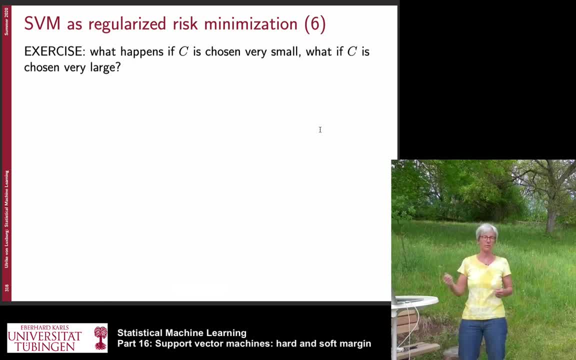 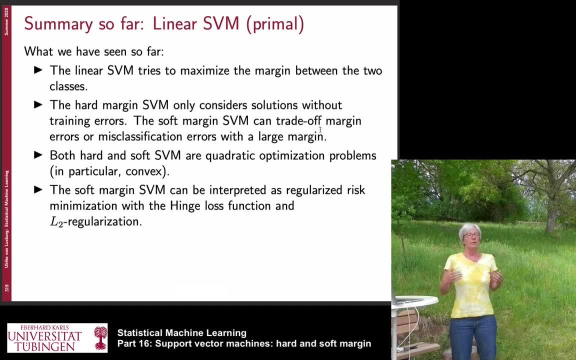 which ones do we overfit? which one controls variance and bias term and all these kinds of considerations. So here's our first summary. We have seen the linear SVM and what we have seen is the linear SVM tries to maximize the margin between two classes. In the hard margin case, we only 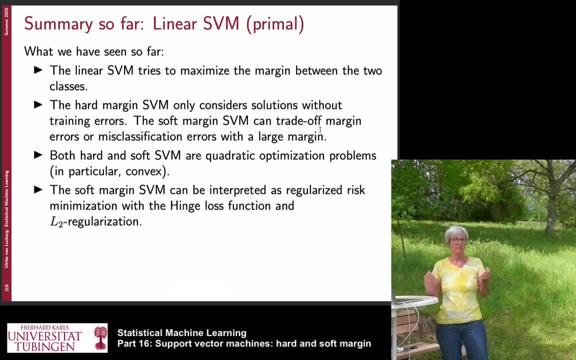 consider solutions that are less than or equal to 1. So we have solutions without any training errors, but the soft margin, SVM, can look at these training errors and has sort of a trade-off between the errors of your solution and the margin. In both cases, both for hard and soft SVM, you end up with a quadratic optimization. 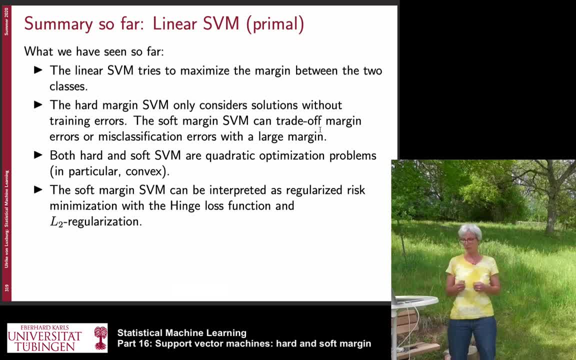 problem. It's convex. it's very nice there exist specific solvers to solve that And we have this interpretation in terms of regularized risk minimization with the hinge loss function. So I don't know whether I mentioned the name of this loss function. It's called the Hinge.